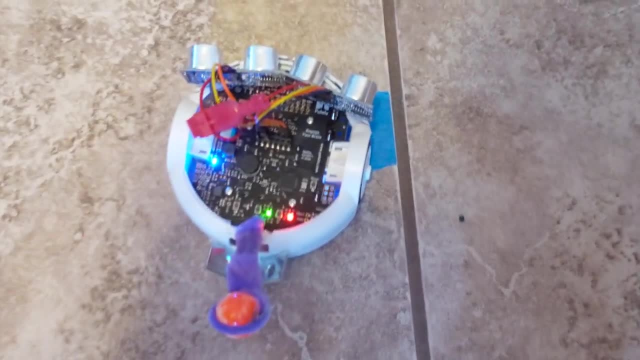 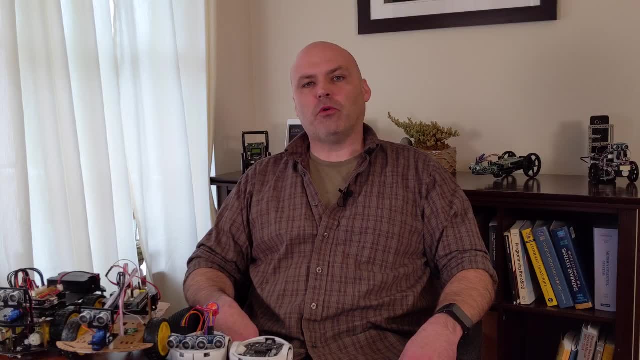 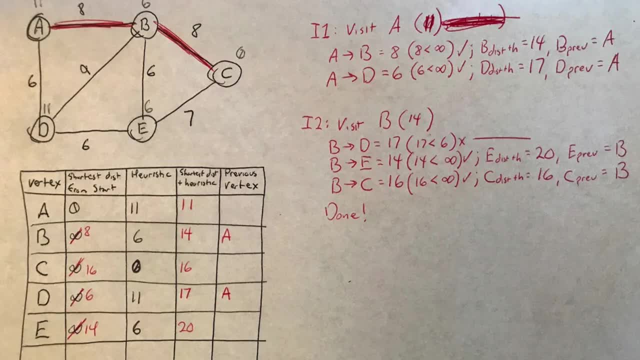 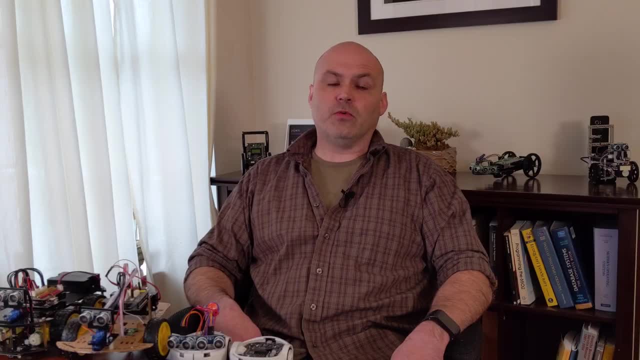 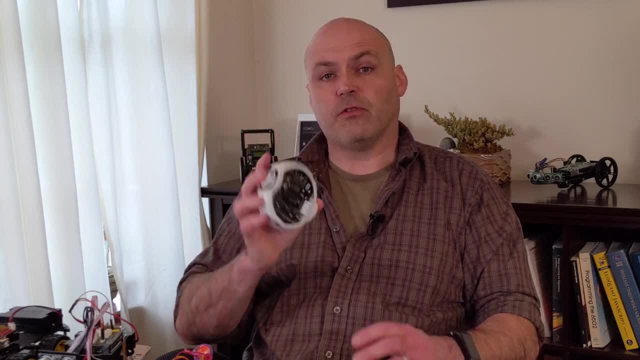 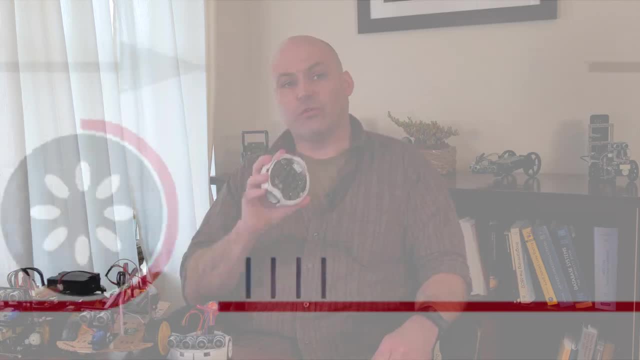 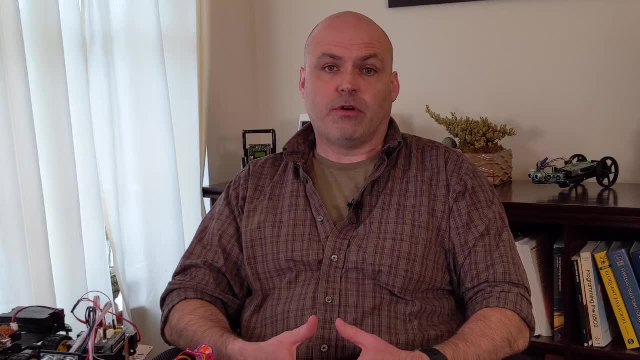 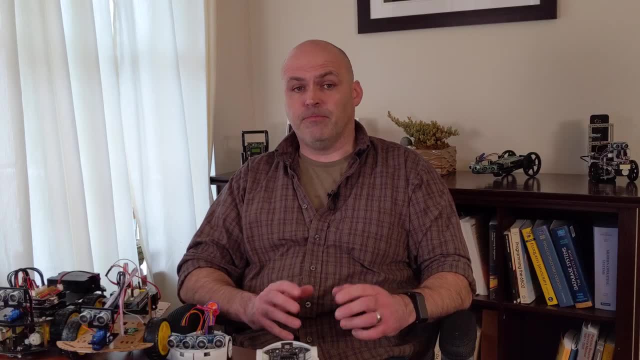 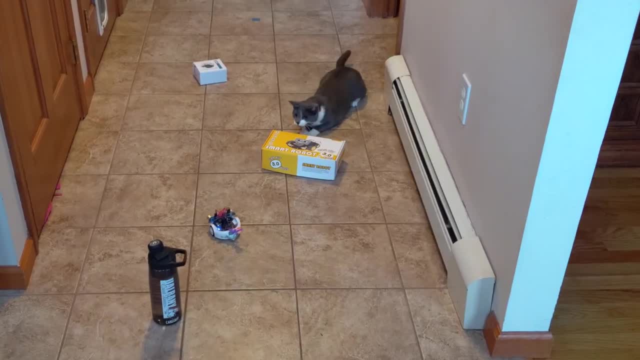 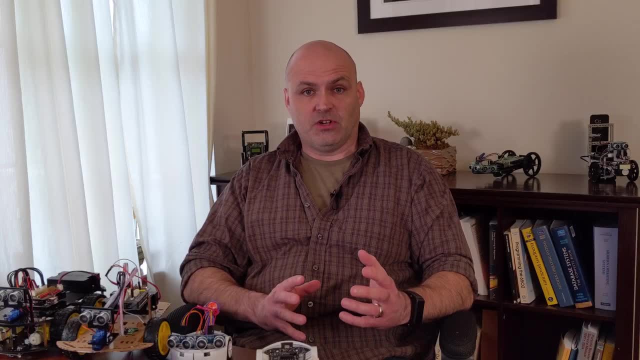 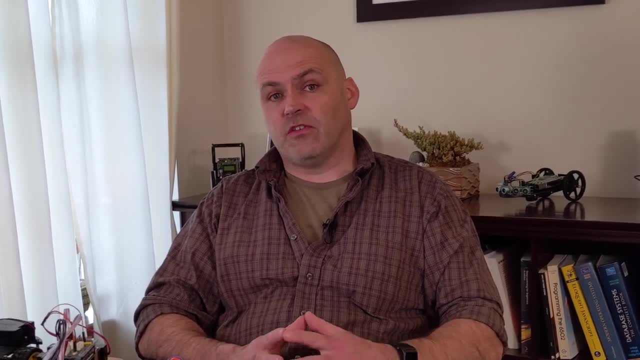 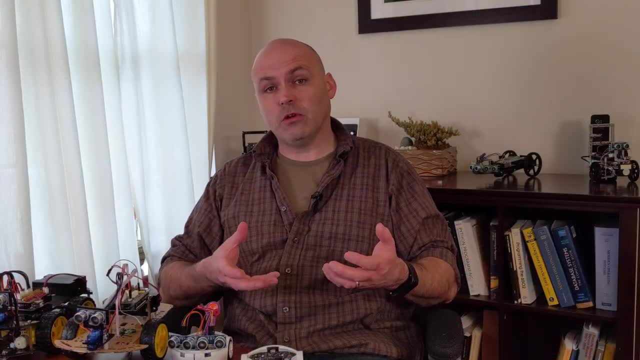 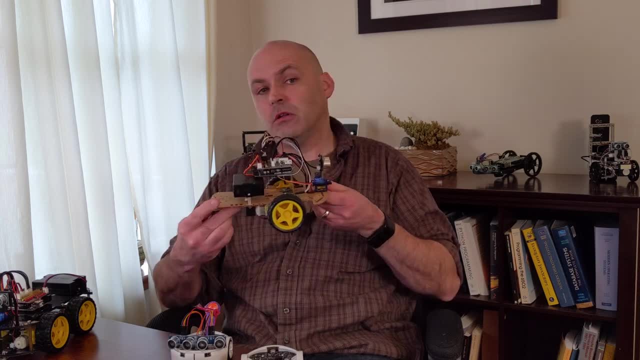 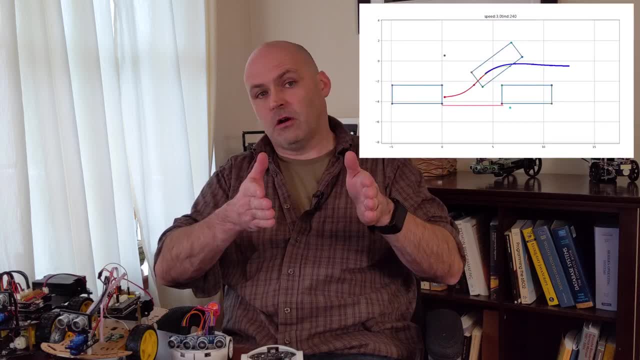 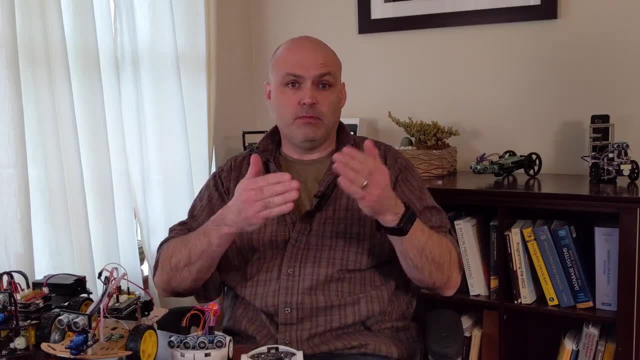 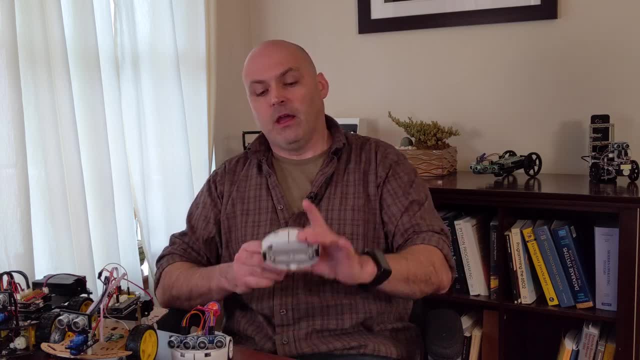 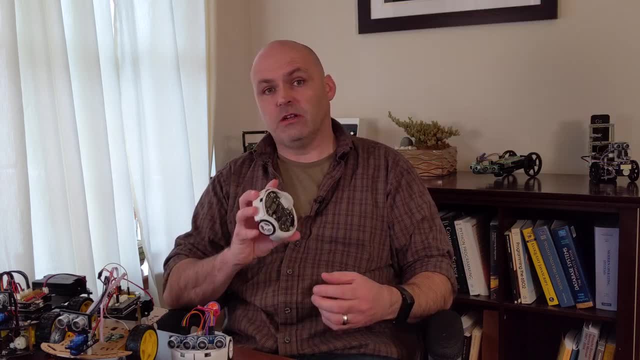 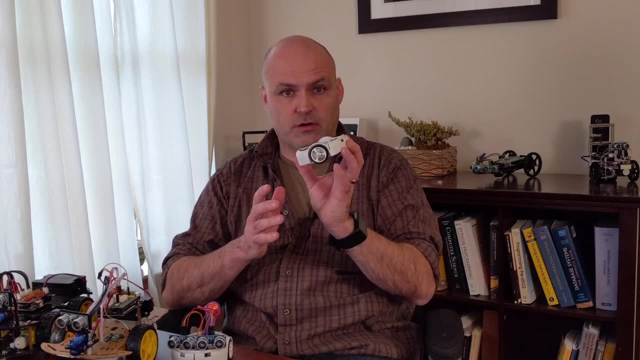 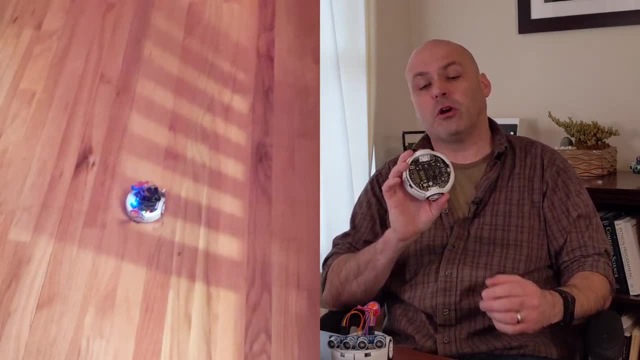 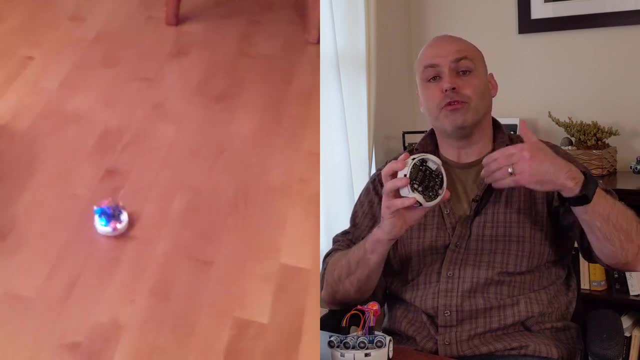 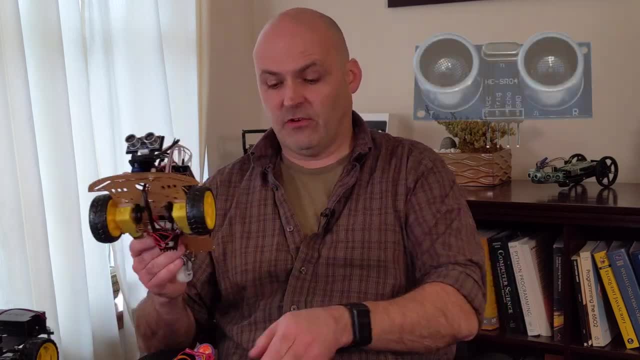 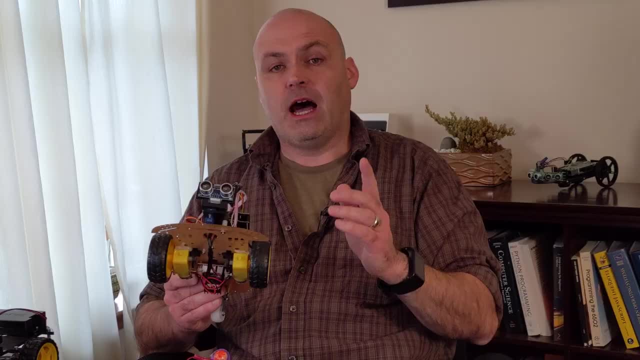 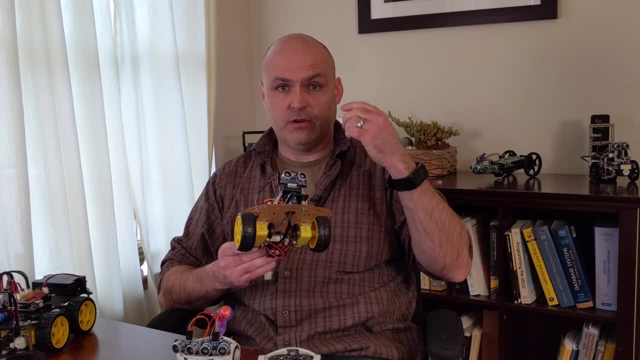 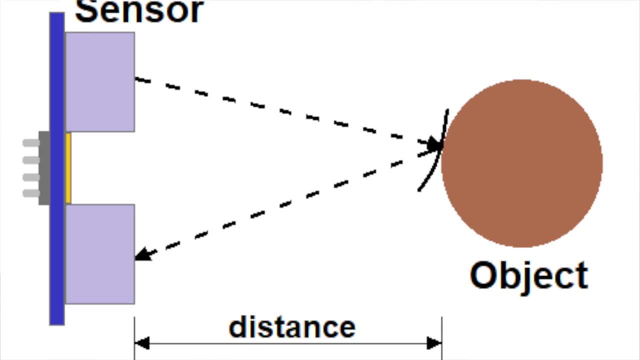 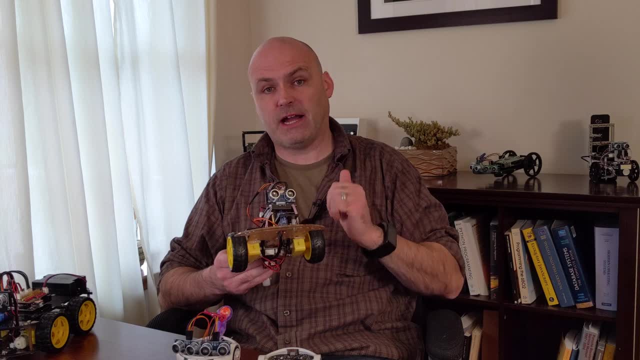 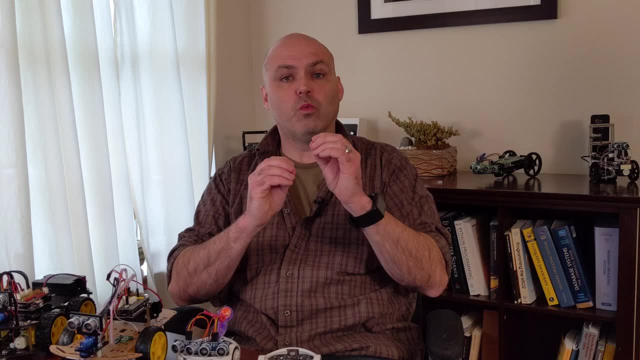 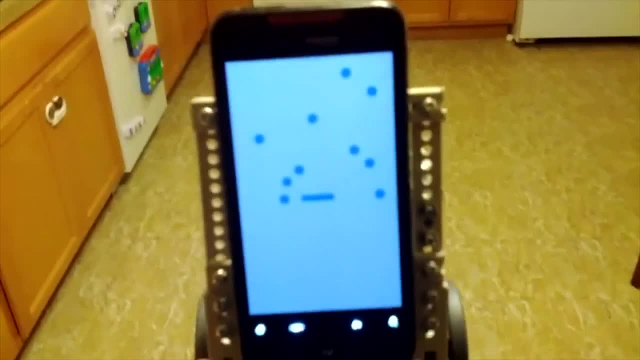 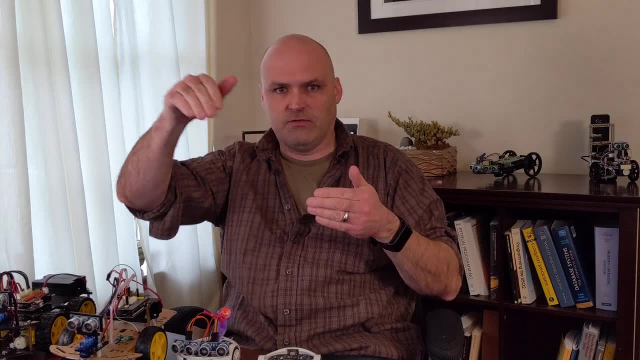 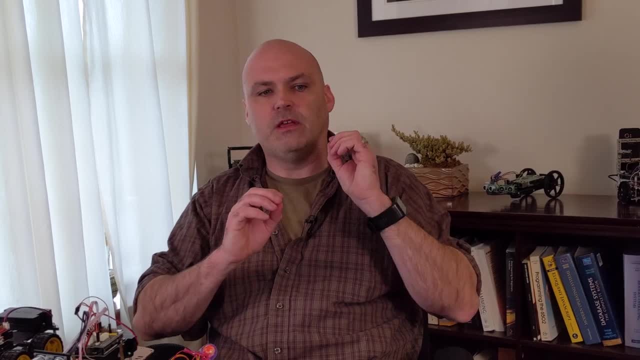 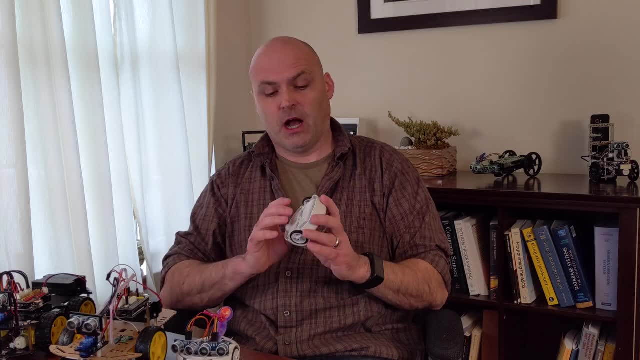 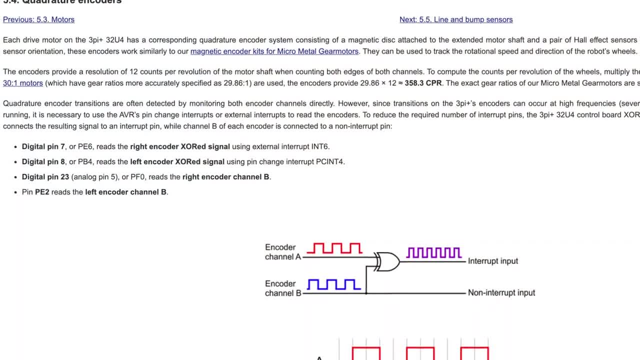 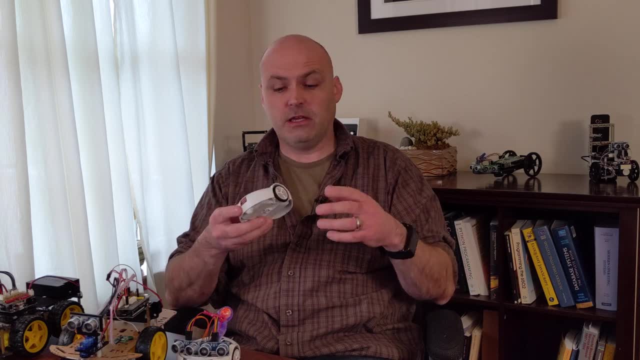 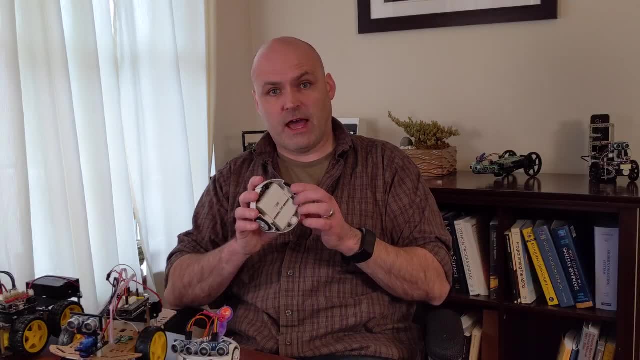 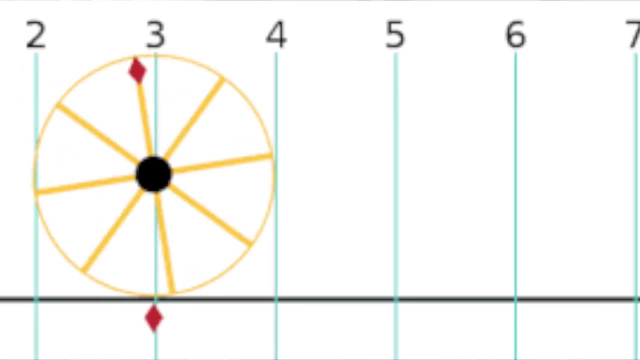 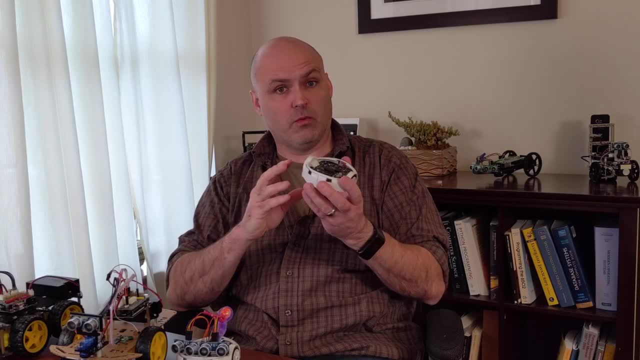 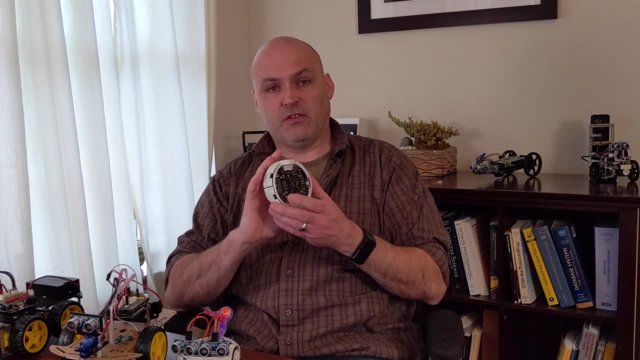 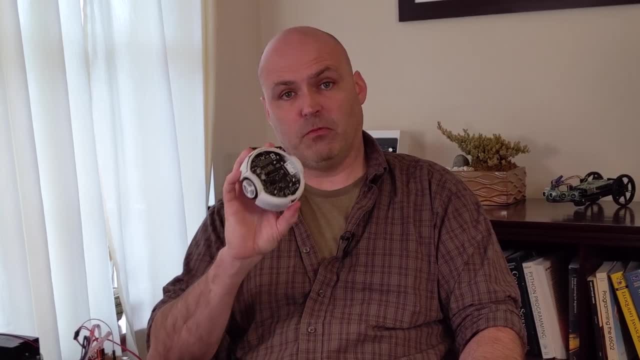 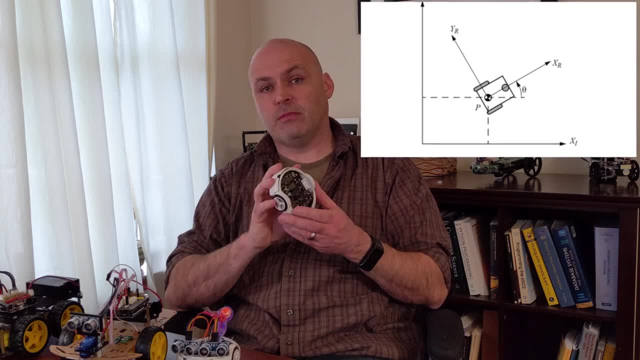 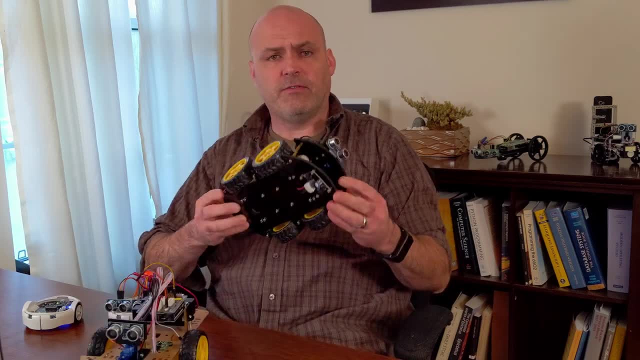 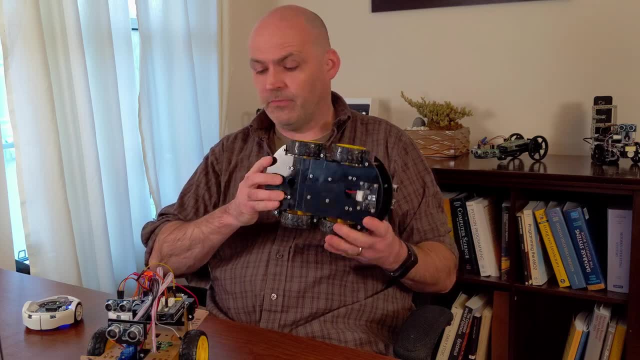 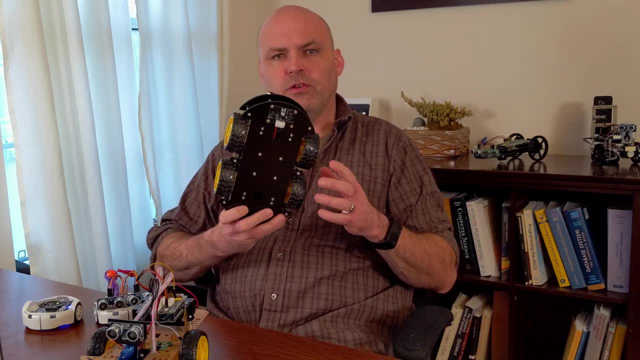 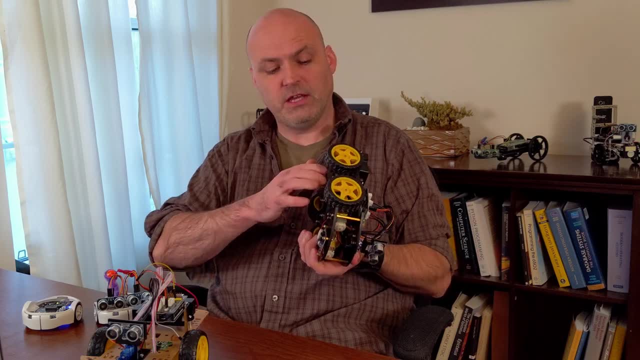 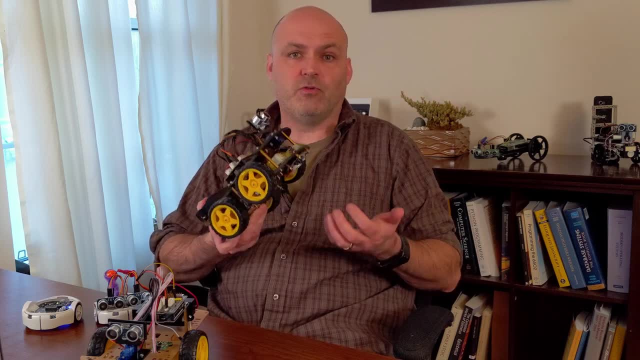 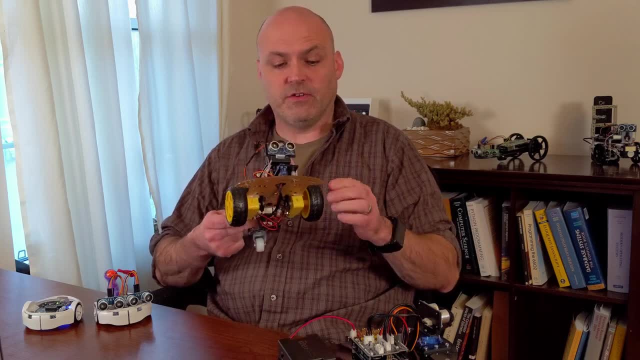 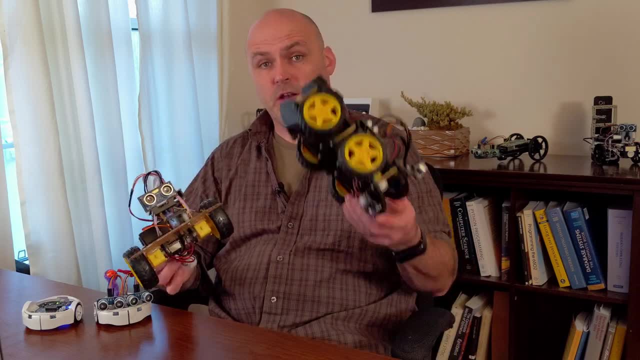 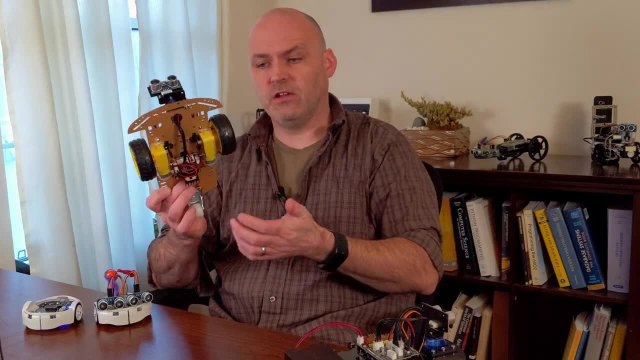 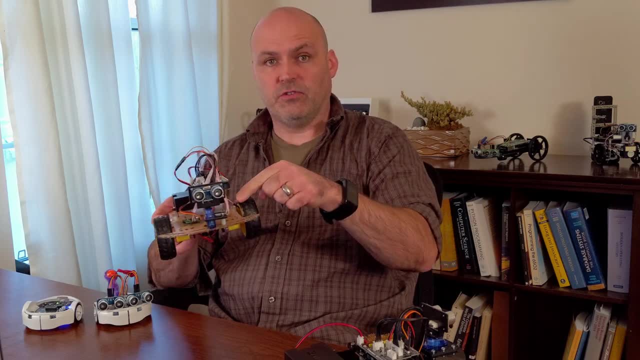 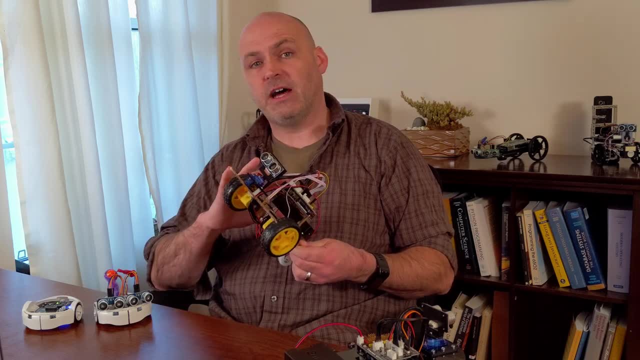 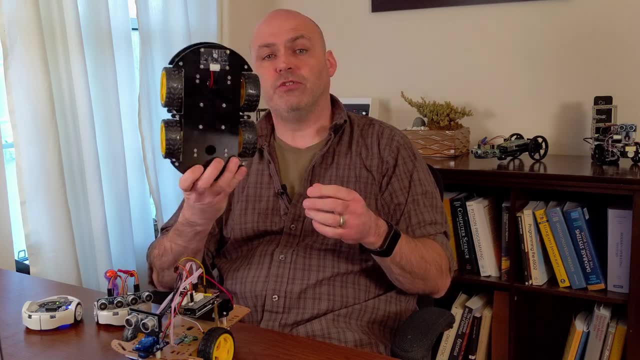 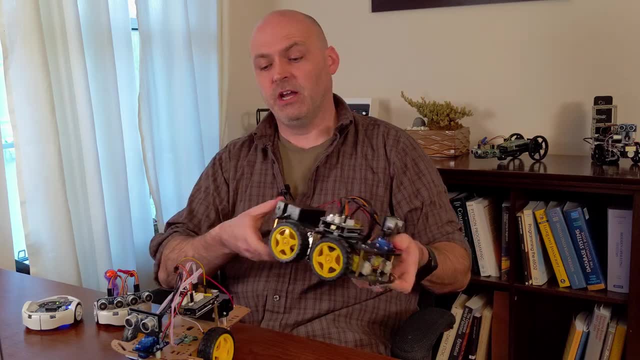 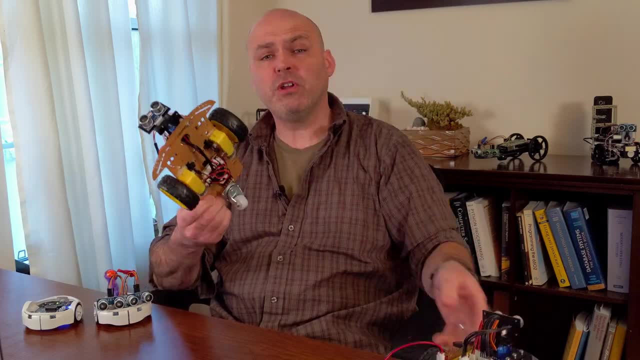 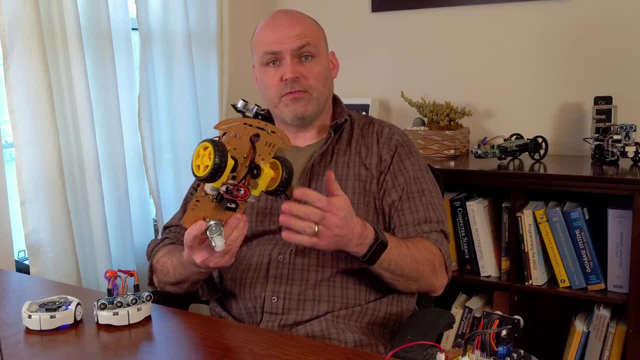 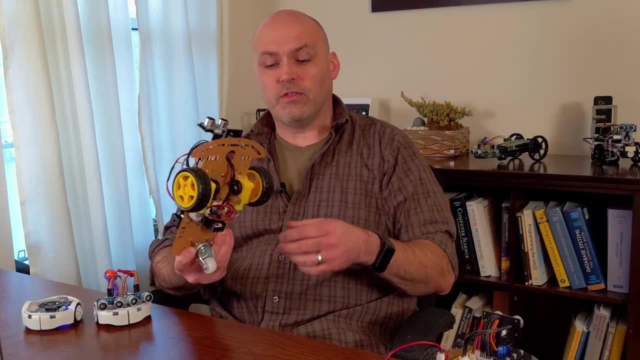 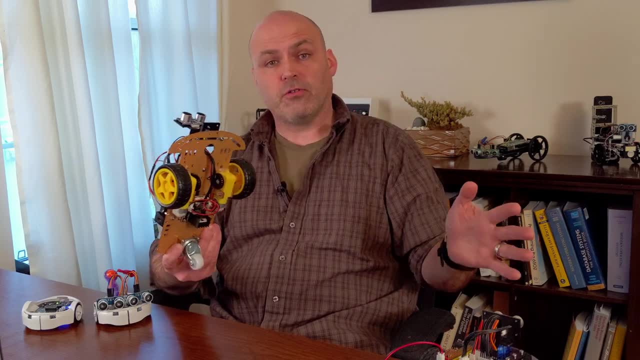 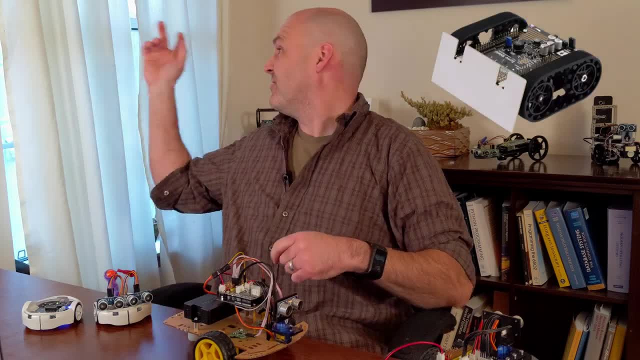 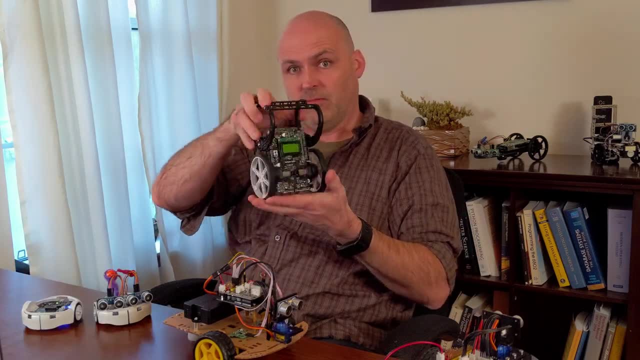 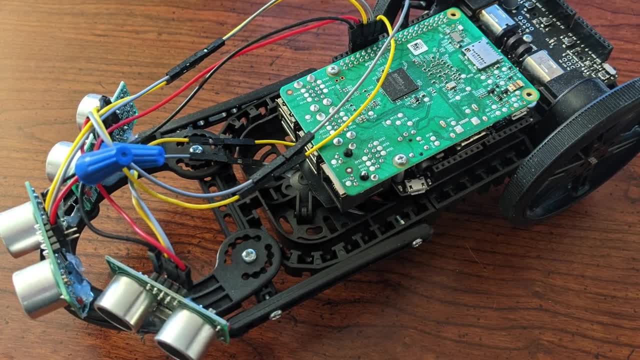 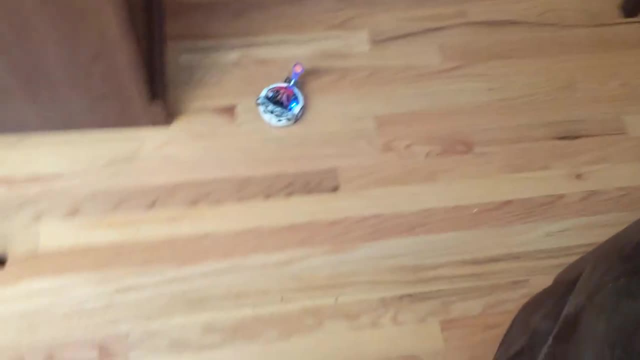 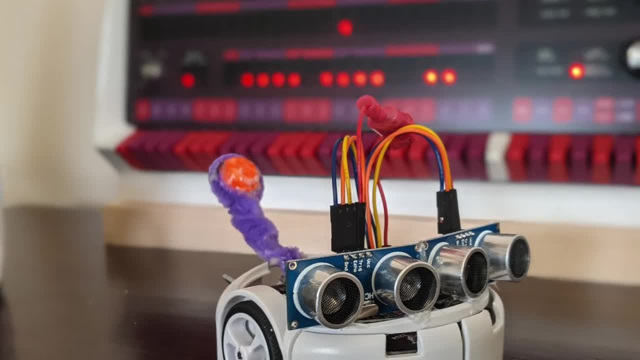 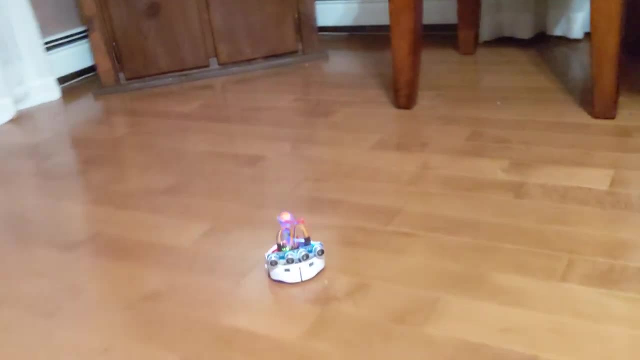 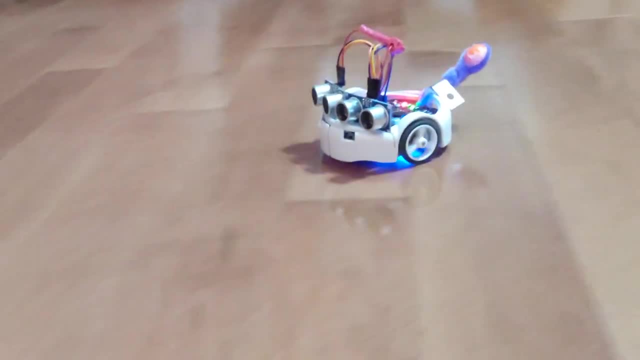 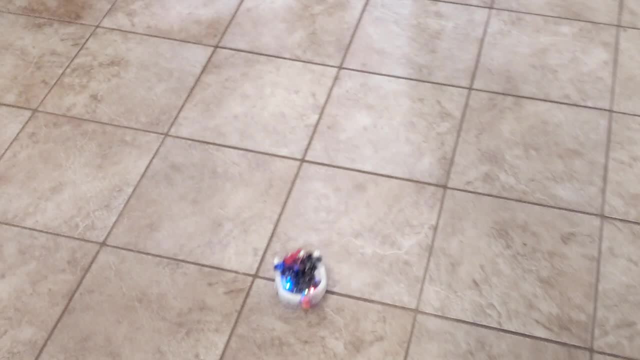 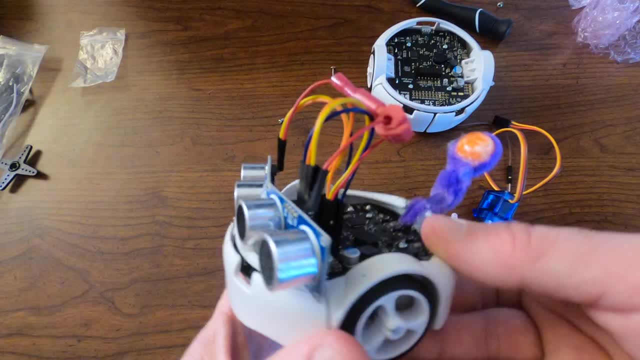 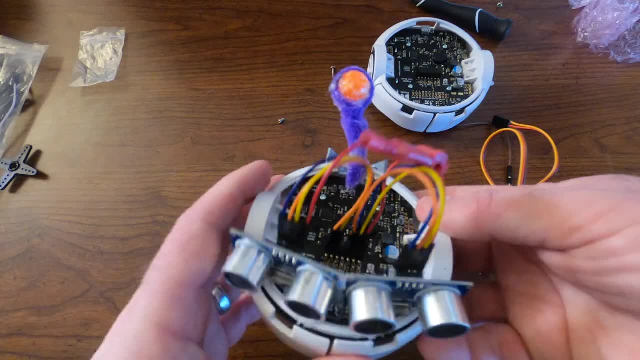 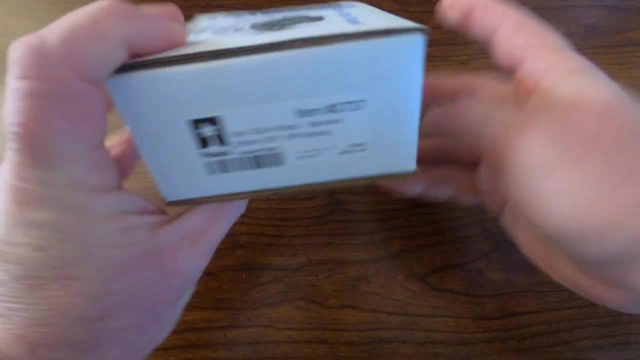 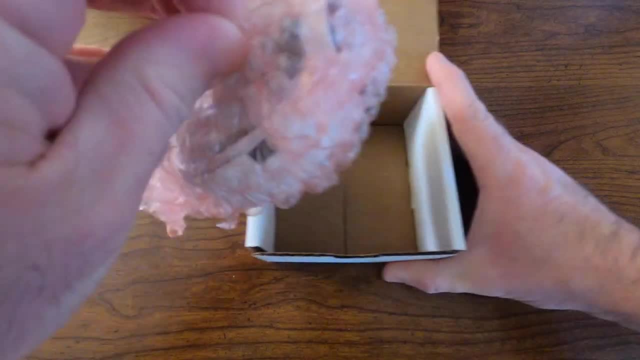 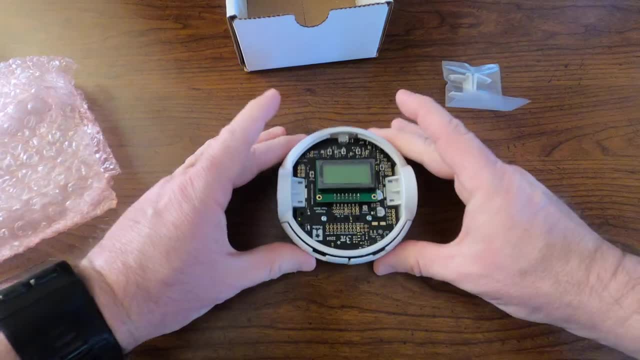 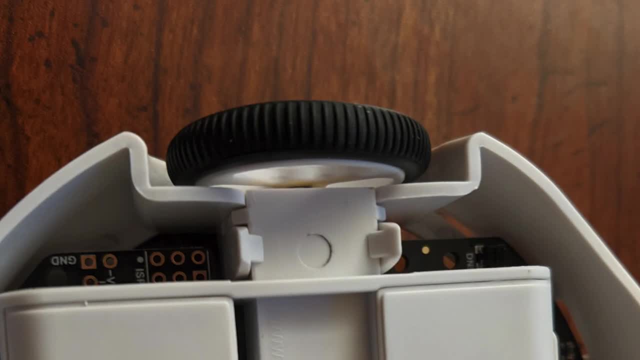 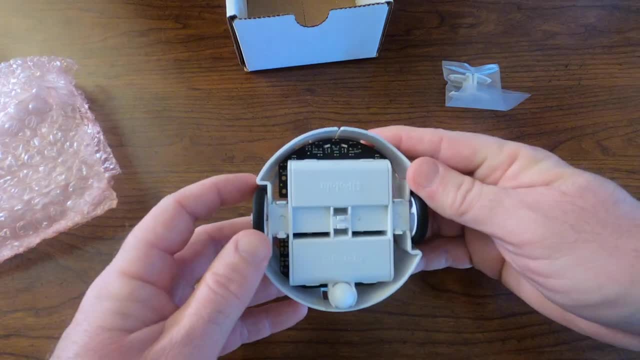 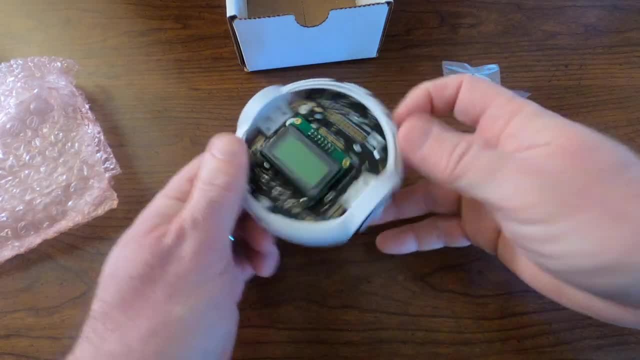 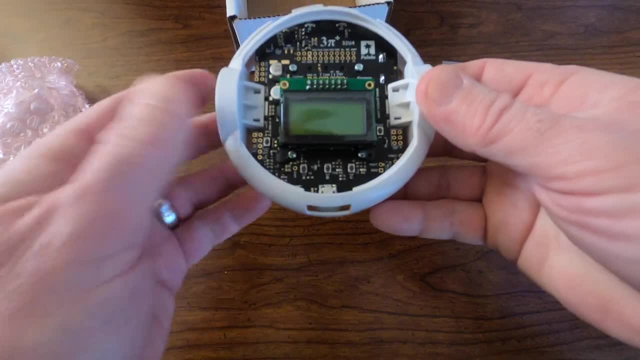 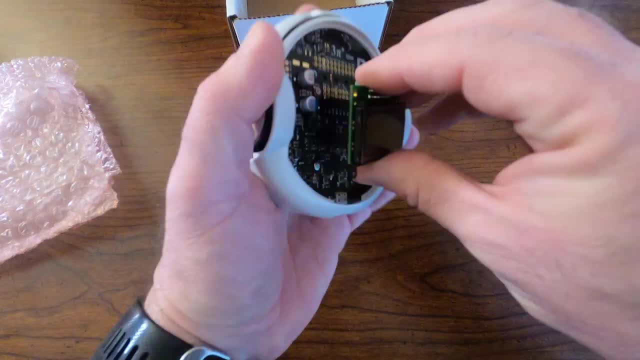 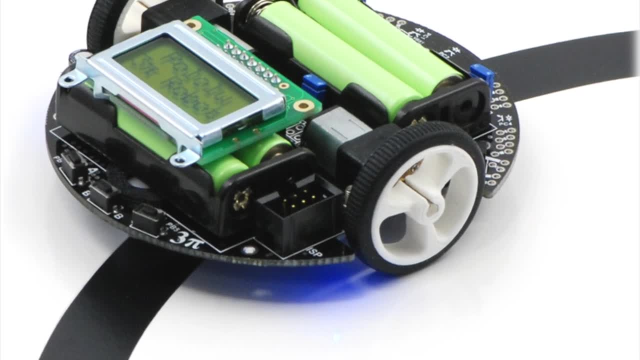 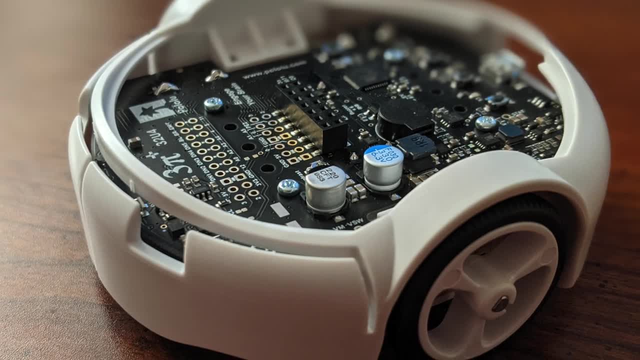 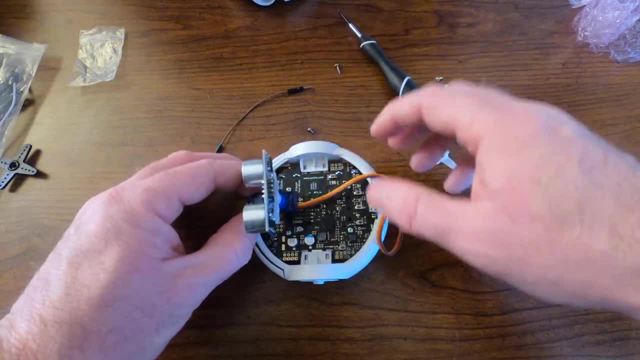 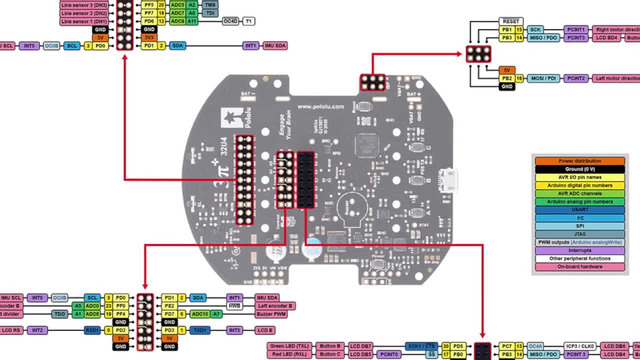 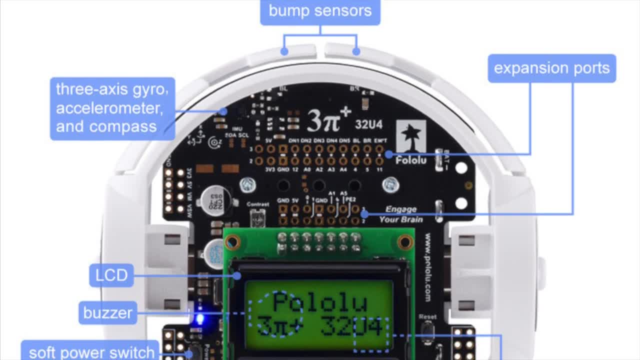 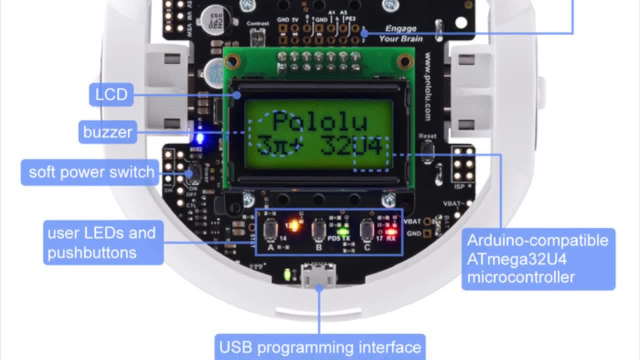 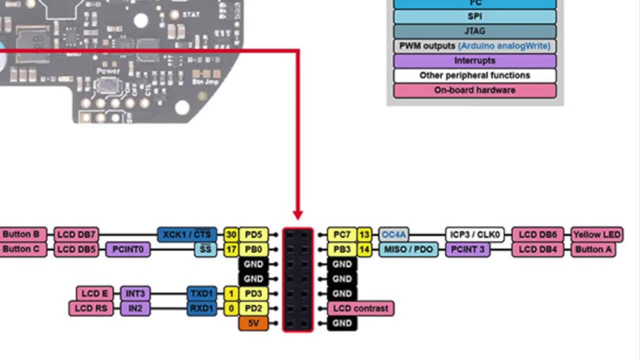 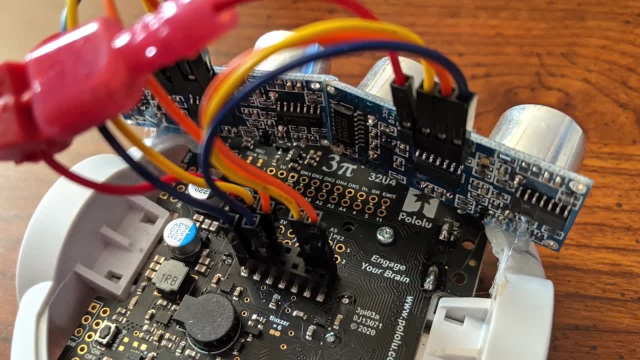 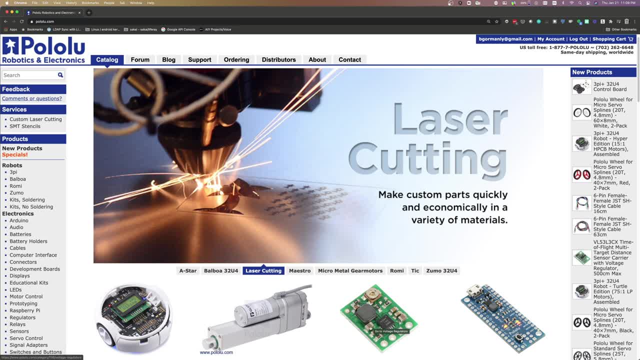 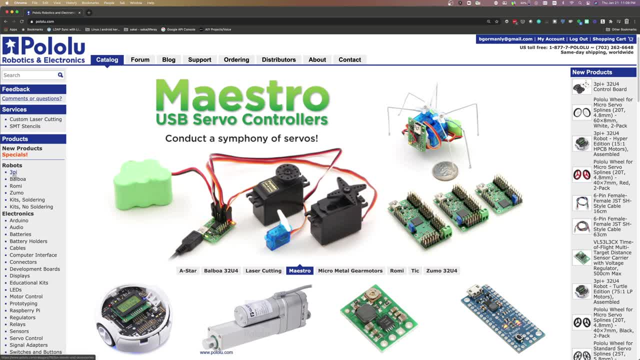 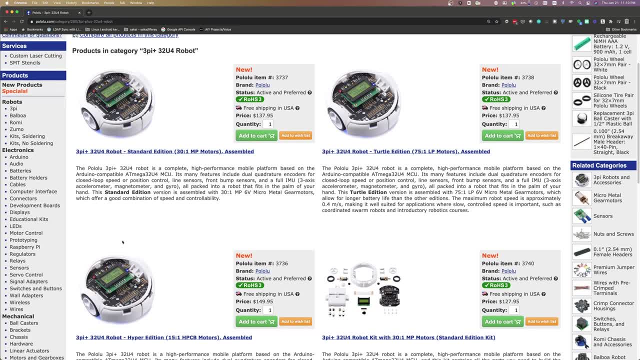 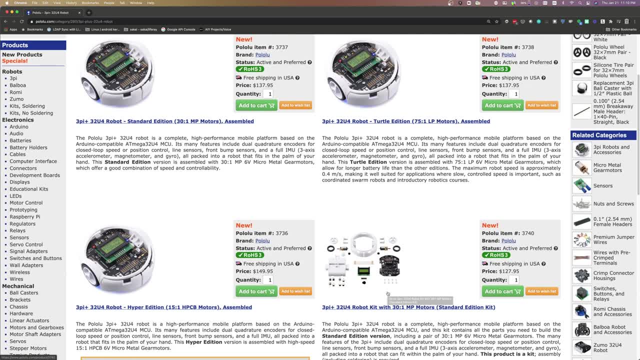 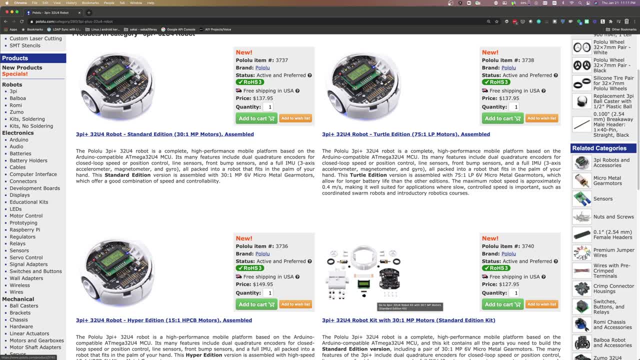 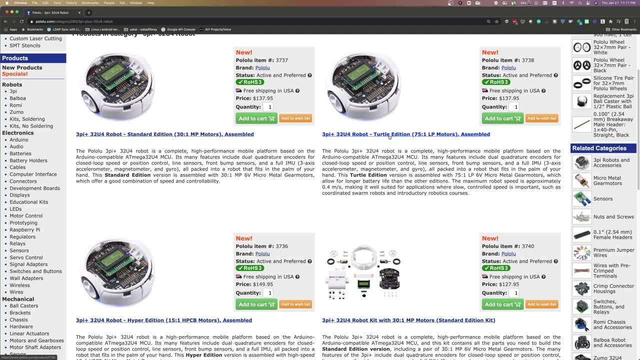 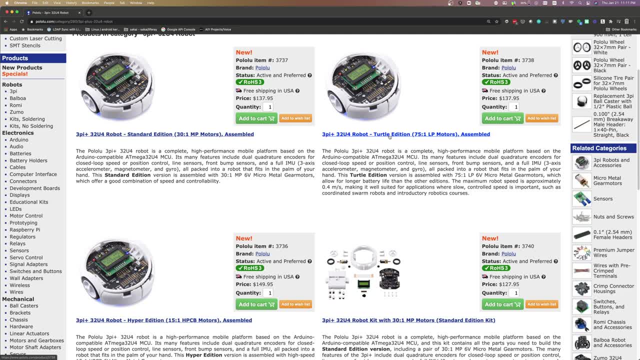 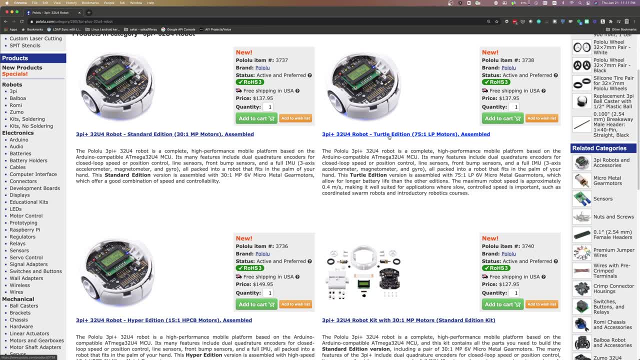 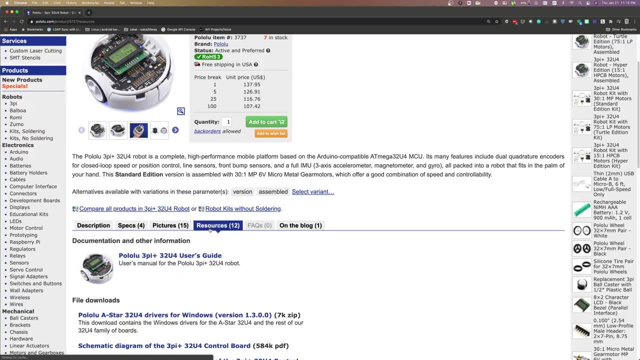 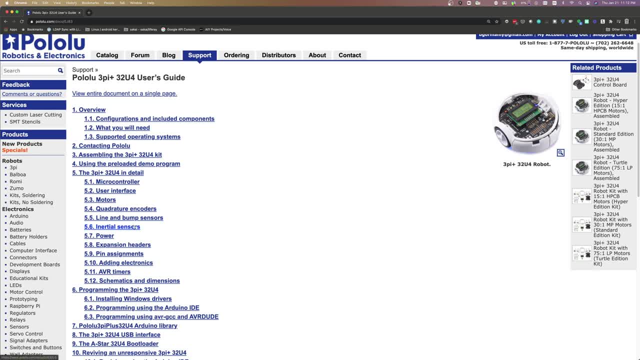 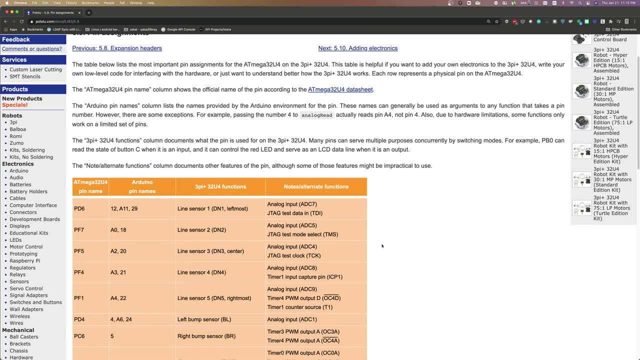 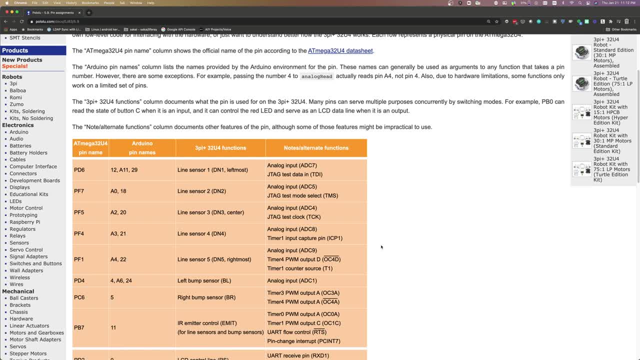 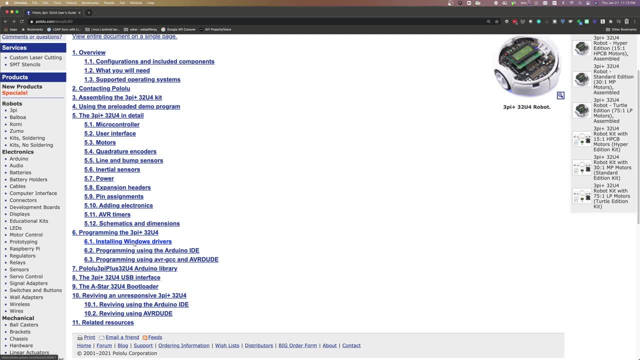 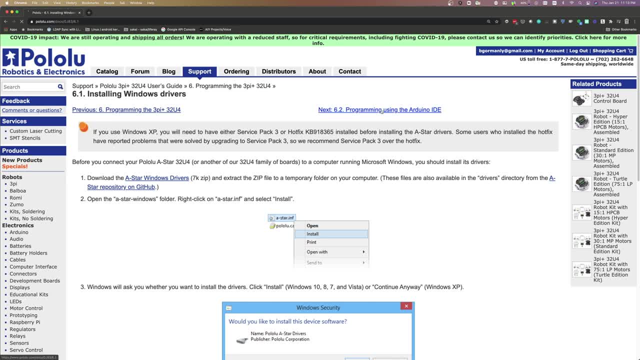 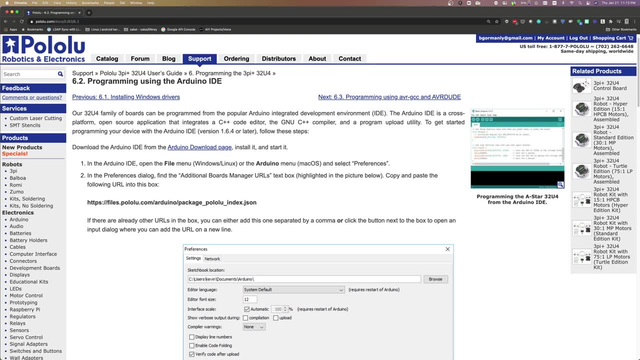 Please subscribe to the channel and press the bell icon to receive notifications when I upload a new video. Thank you for watching up your Arduino IDE in order to work with the 32U4.. Now the 32U4 has a specific software that. 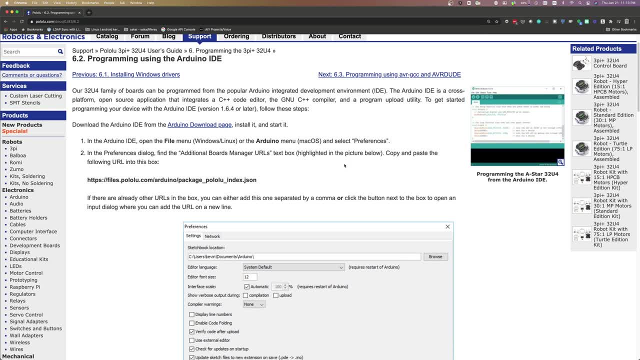 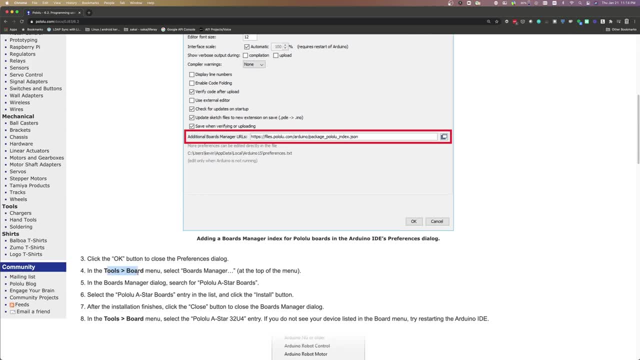 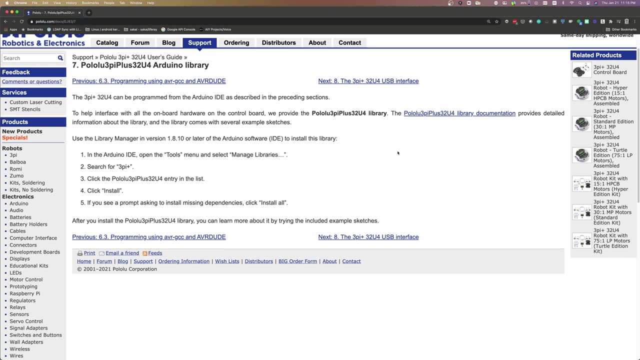 is provided by Pololu, that you can follow this guide to download and install, at which time you will be able to then see those boards in your tools boards menu and select the Pololu A-star board. Another important step is to install the Pololu 3Pi Plus Arduino library. This is 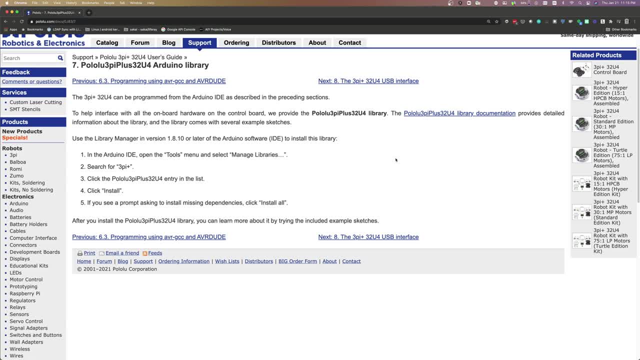 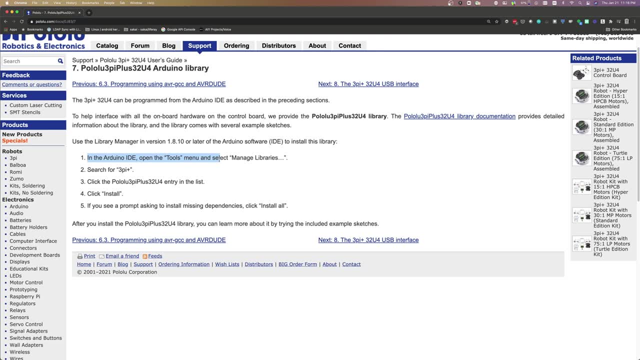 a library of code that's been made available by Pololu to help with low-level control of the hardware. In order to install the library, you're going to go into your IDE, open the tools menu, select manage libraries, search for the 3Pi Plus. Once you've installed this, you'll be able to use. 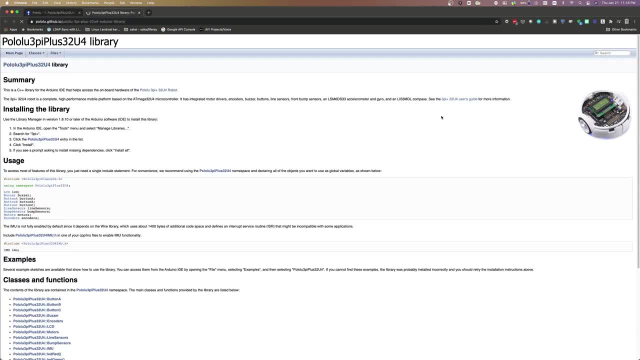 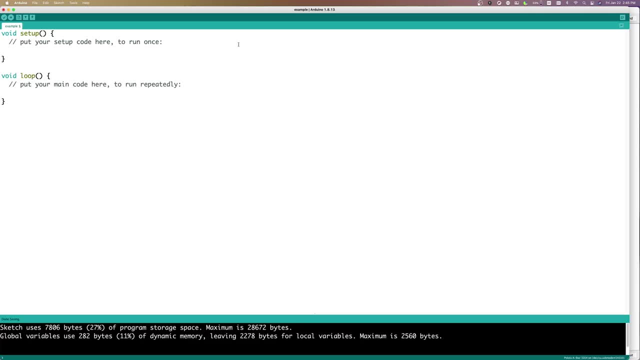 their libraries in your code. Please also explore the library documentation to learn more about the library and how to use it. So, getting started with the code portion now, I've opened a blank skit in the Arduino IDE and I recommend using the Arduino IDE that you install on your. 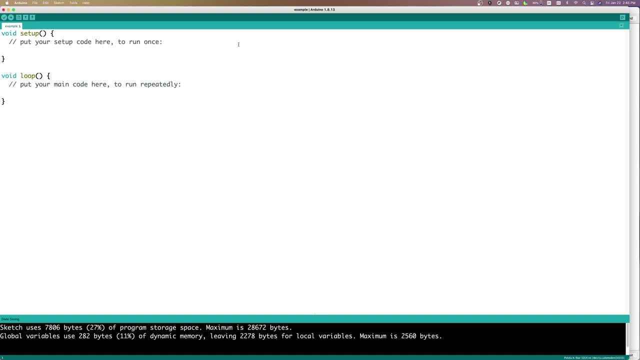 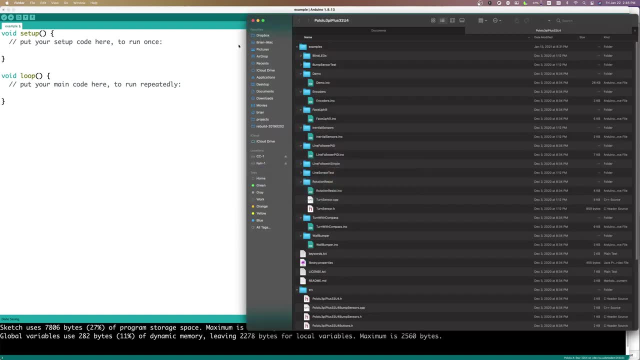 computer and not the cloud-based version. I want to take a moment to just look at the library as well that they've provided. So if I go over to my finder here, a couple things I want to point out is just once we start flashing this device, if you ever want to return it to its stock form. 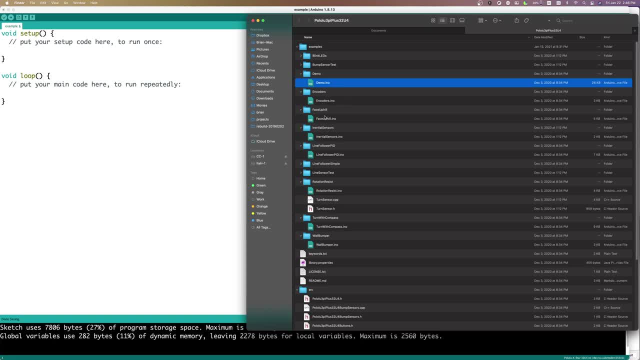 they've provided that demo program here, And there's a lot of other examples programs here that can help a lot when you have questions about working with specific hardware. So, for example, there's an encoders one right here that we're going to use, In fact, while I'm here. 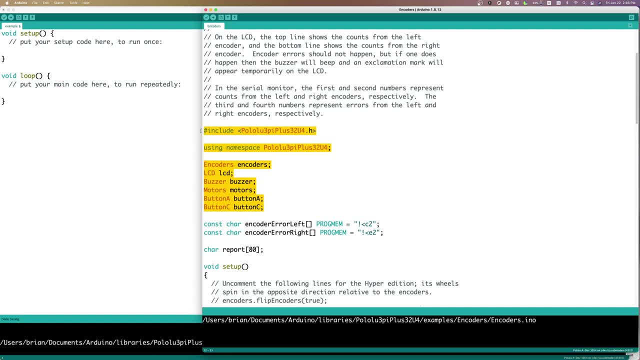 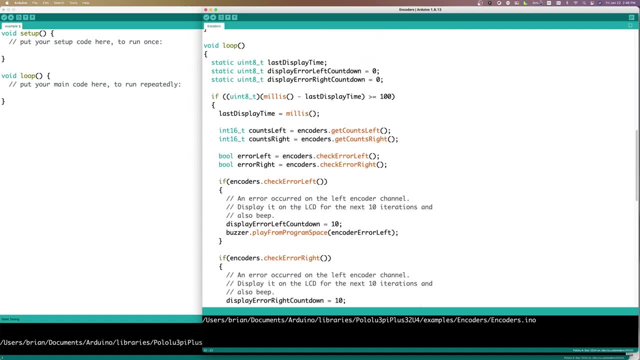 I'm going to grab this code here and I'll describe a little bit more about what this code is as I paste it in, but it's going to save me a little bit of effort as I do. I want to just note, too, that I'm not going to follow this verbatim. However, it is worth coming back here and 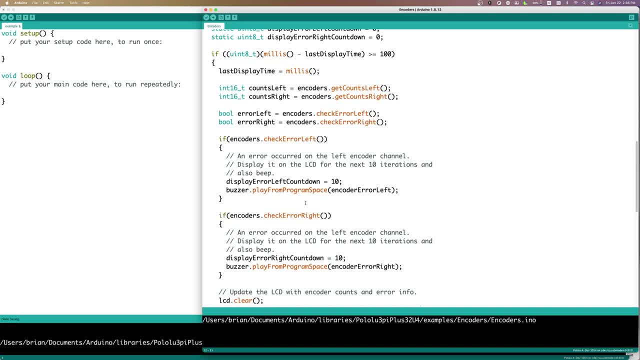 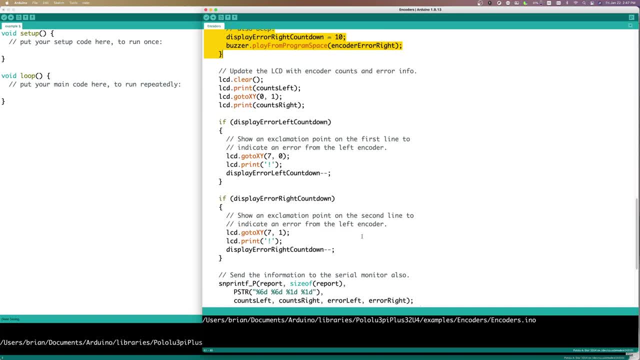 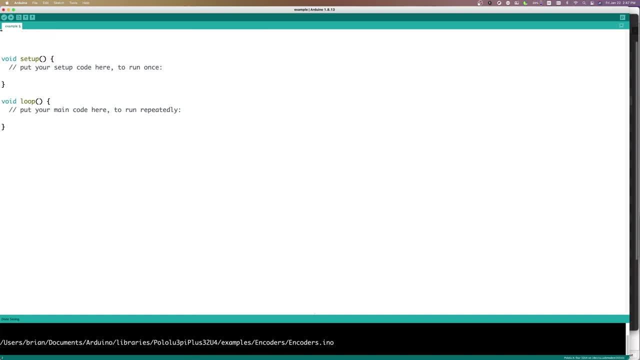 there's a good example here of exactly how you should do that. All that said, I'm going to just close this and we're going to come over here to our own skit And we're going to paste in this code. You can, of course, you know, type it in or get it from any of those other examples. 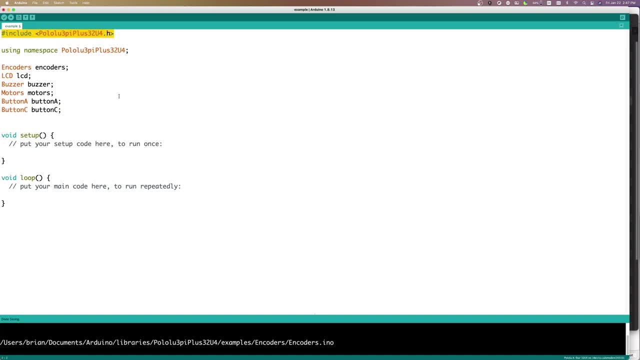 But what we're doing here is we are including that library, the Polu 3Pi Plus 32U4 library, and the namespace that goes with it, which then allows us to just refer to the classes within that namespace. Now, these are different pieces of hardware that we intend to use and we're using. 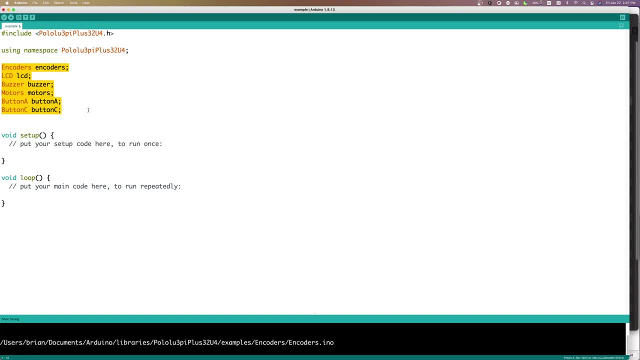 their library in order to avoid having to write that low-level code ourselves. For today, we're very specifically going to be working a lot with the encoders. I actually don't need the LCD, so I'm going to remove that. I will, however, be using the buzzer and the motors, and at least one. 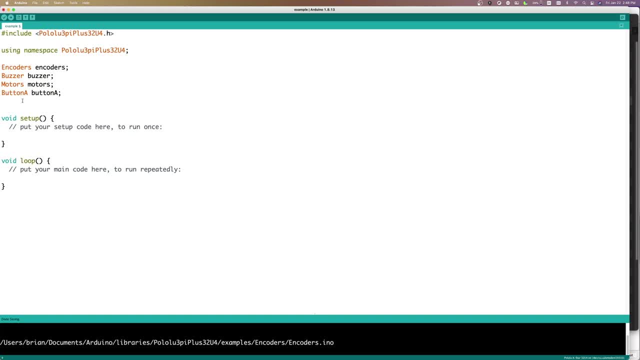 of the buttons, I think I'm going to remove button C because I don't foresee using that. To get started, I'm going to go to setup here, And it's worth noting in case you're not familiar with Arduino: setup runs once when you either start the device or reset it. So basically, 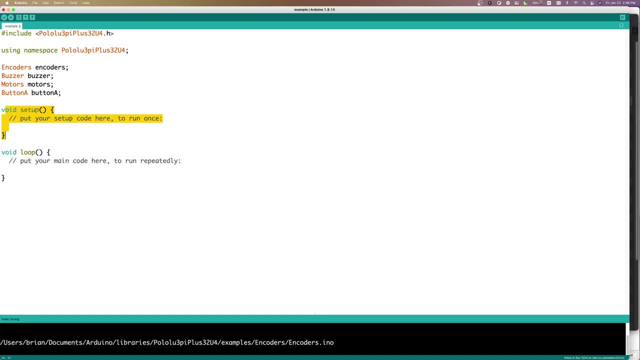 when power is applied or a reset is applied, you run setup once. Then the loop continually runs throughout the life of the program. One thing that I want to set up is my serial connection so that I can use my serial monitor. So we do that by typing serial begin and providing a baud rate at which we want to send information. 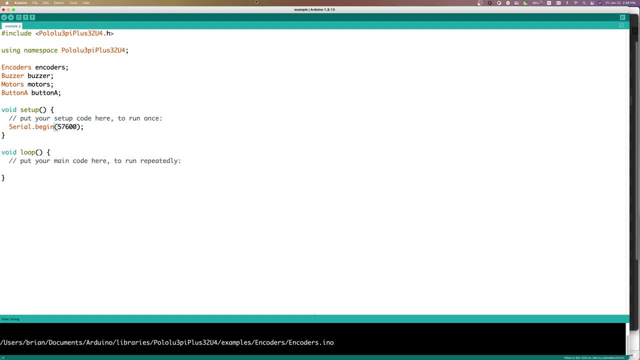 to the serial monitor. I will show this on the serial monitor in a few moments when I actually use that to display some output. So for right now we're going to leave that like this. I'm also going to add a delay here Now. I normally recommend against delays in general. However, 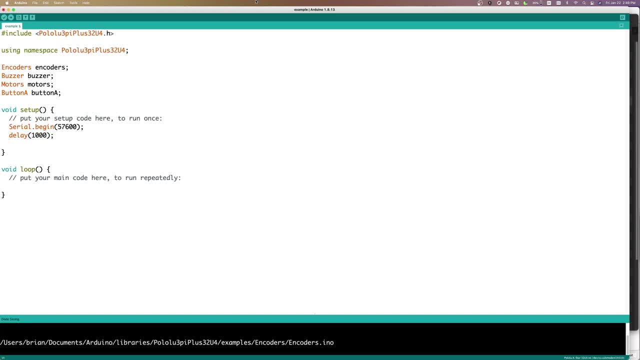 in this rare instance in setup, I do like using it Oftentimes. although there's not at the moment, there's some hardware that might need to calibrate and the delay provides for that. But I also like to just have the robot wait a second before it runs away when I say press reset or something. 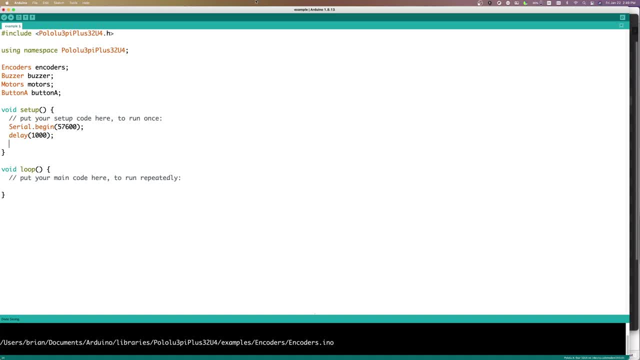 like that, So I've just gotten in the habit of adding a second delay there. Another thing I want to do is I want to have this thing play a note when it's starting, just so I can audibly hear that, yes, the robot is kicking off and I know that that means that I am on my way and running. 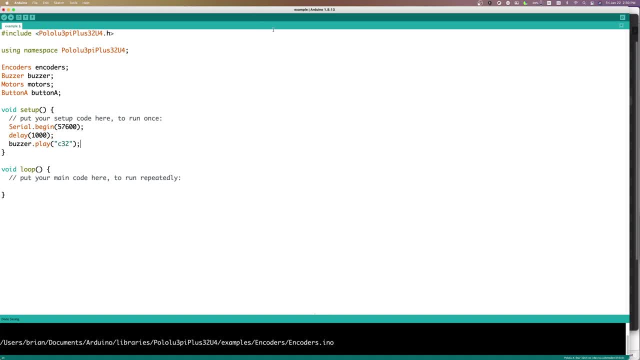 through the system. It's just more to appease the human who is coding it, to kind of know that things are happening, than anything else. So that's all I really need there for now And for this very first deployment. we're going to keep things super simple. I'm not going to bring the encoders in, just. 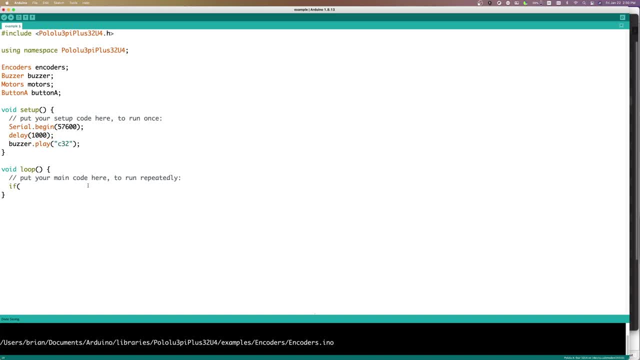 yet I just want to put some code in so that we can see the motors work. But to make it so the robot just doesn't run away endlessly. I'm going to make it so that the motors will run if we press button by using the button that is provided there. Button A is the button that we've brought in And we're 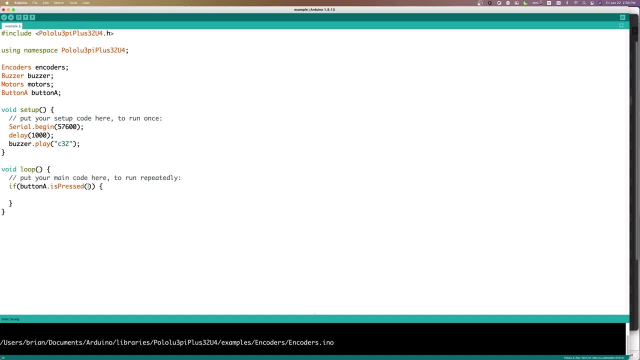 going to use the is pressed method, And when we press the button we want the motors to run. So to do that, we have motors and set speeds is the method that we're going to use And I'm going to set mine. 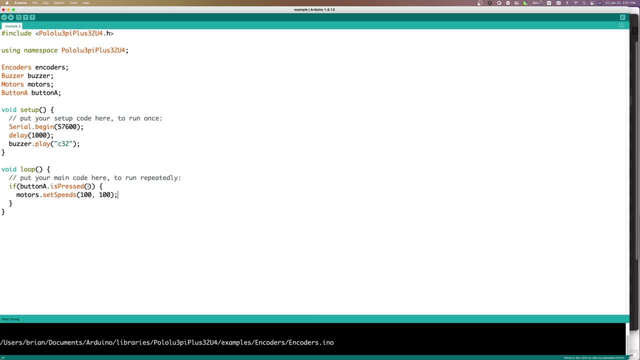 to 100.. I have the standard edition. If you want to try it a little bit higher than that, you can. If you have the turtle edition, you could go higher than that for sure. If you have the hyper edition, I would actually recommend going slower than that, Anything less. 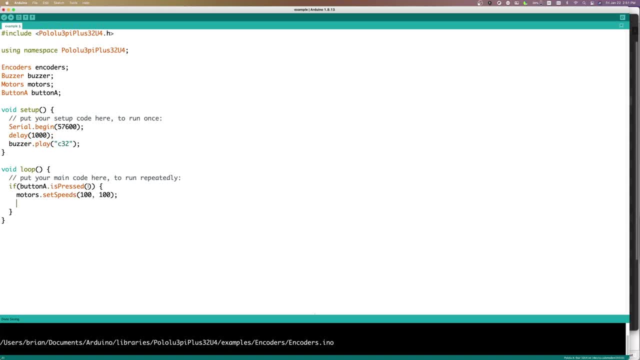 than you know. 50 is questionable for stalling. Definitely say less than 30. It depends on the motors themselves and the gear ratios and things like that. But don't expect the motors to be moving if you only provide a very low value of, say, you know less than 30 and possibly even less. 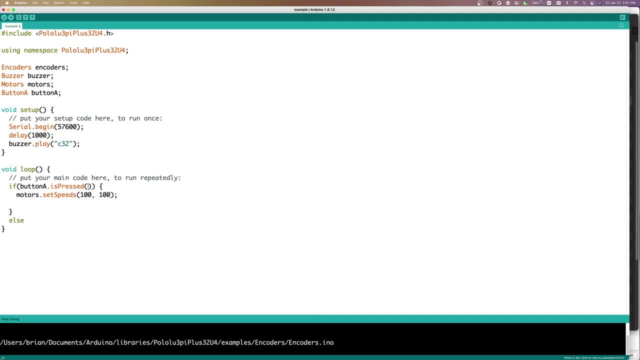 than 50 could be a problem. Now, the only other thing we really have to do here is make sure the motors are not running When we are not pressing the button. So I'm going to provide an else here and I'm going to set the speeds. 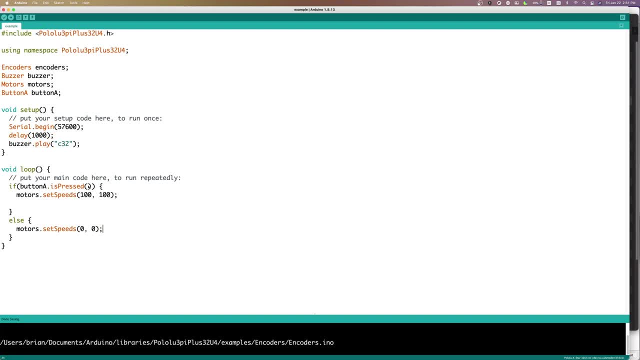 to zero when that is the case. So I believe this is pretty well done. The only thing I want to do is I'm going to add something here for the serial monitor more so that it can show exactly how that works and you can get used to using it. So to do that, you do serial print And if you do print with 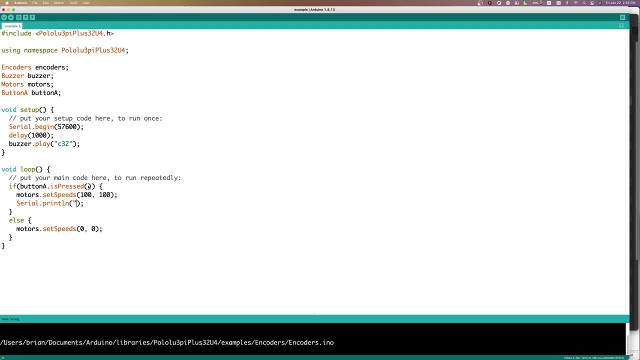 LN, it'll do everything on a new line. So what I'm about to type here will get a line of its own, And then the next thing that gets output will be on a separate line. If you leave off the LN, it will just keep putting things on the same line You're going to. 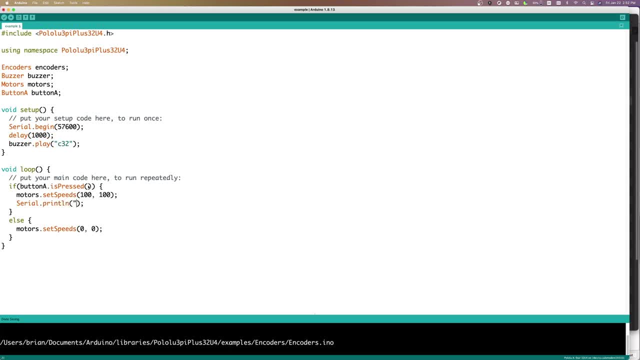 want to do that later, as you can't really concatenate in here very easily. For now, we just want to know that our motors are running. So let's say that: So motor's running and we are good to go Now. you have to usually save this before you run it, So go ahead and do that And you also. 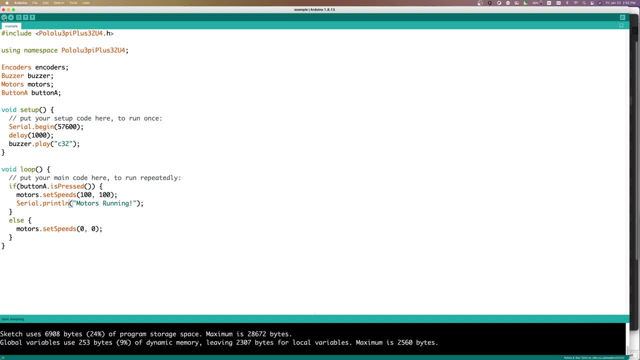 should check it with a verify. So what we're going to do is we're going to go ahead and do that. So we're going to click the check here. It's going to compile the sketch. It says: done compiling. It looks like everything is good. I'm going to bring over my serial monitor here And I want. 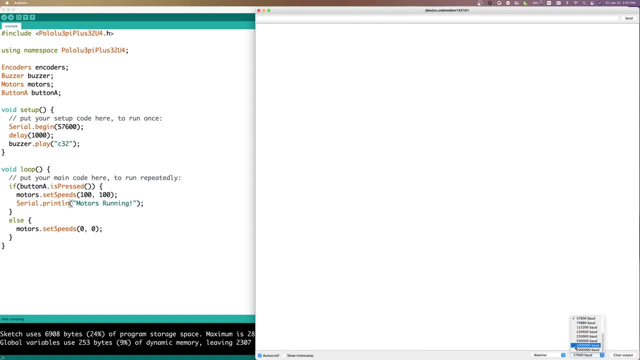 to point out that it's at 57,600 baud, So that matches what we have here in our serial begin, which will allow communication between our computer and the robot. At this point we're ready to go to try this out Now. one thing I want to note is that your motors will not run. 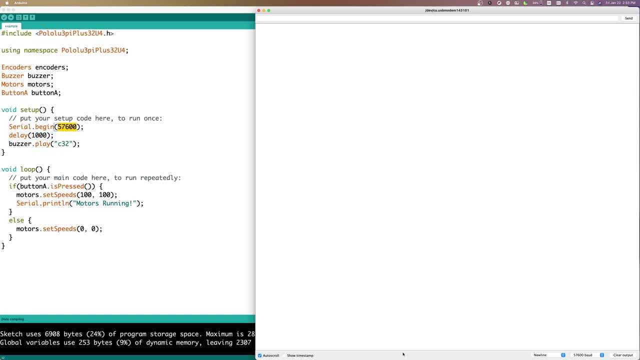 if your power on the robot is not on, If you just plug in USB you will have power enough from the USB connection at 500 millivolts to power the actual 32U4 chip and the electronics. But the motors themselves only run off of battery power. So the little power button that's on the kind of 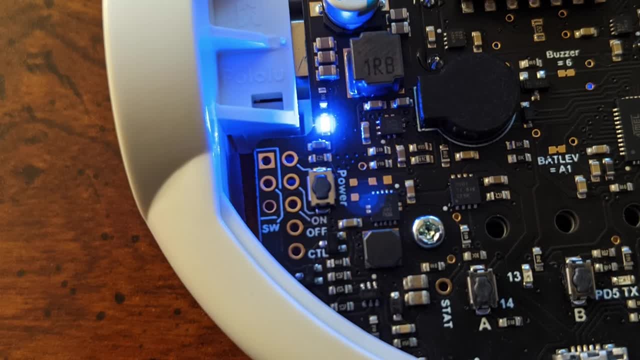 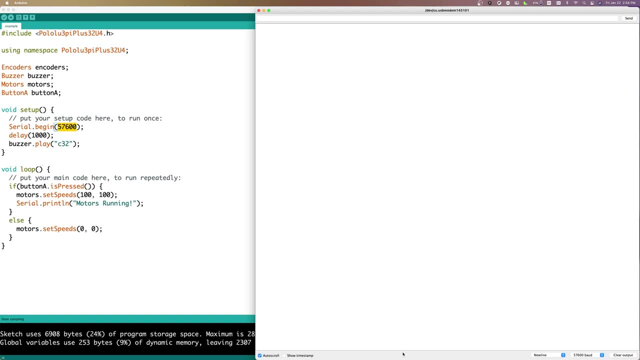 bottom left-hand quadrant of the robot. that needs to be pressed And the blue light that's directly above it needs to be on in order for your motors to actually start running. So we're going to spin. You can upload programs and run them without your motors being on or your power being on. 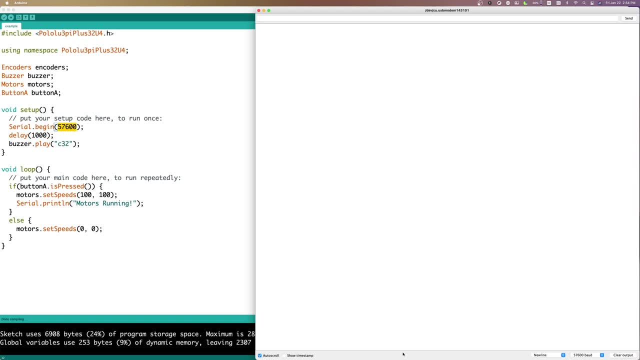 I should say as long as the USB is plugged in, But be aware that things that require the extra power, like your DC motors, will not be running. To deploy this now. I click the upload and it says it compiles the sketch and it uploads. I should hear my beep. 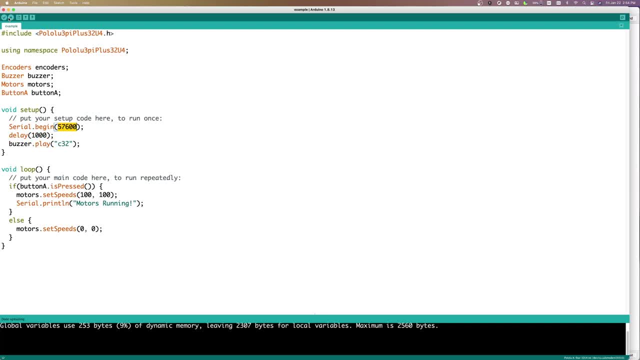 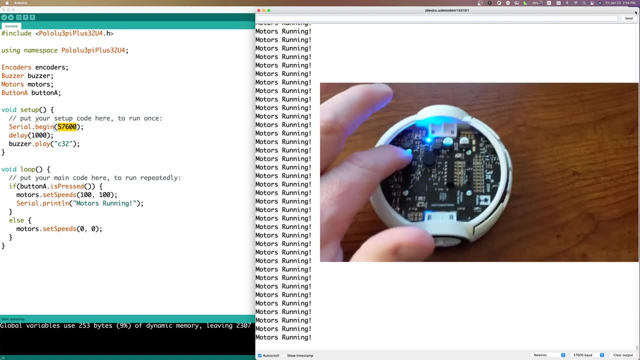 There it is, And now that it's on, my power is on. I should be able to press A: Let's get our serial monitor ready here. There you go. You can see that- all my motors running up here, And if I clear, 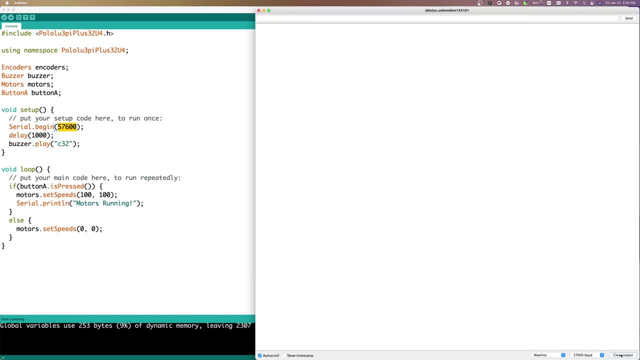 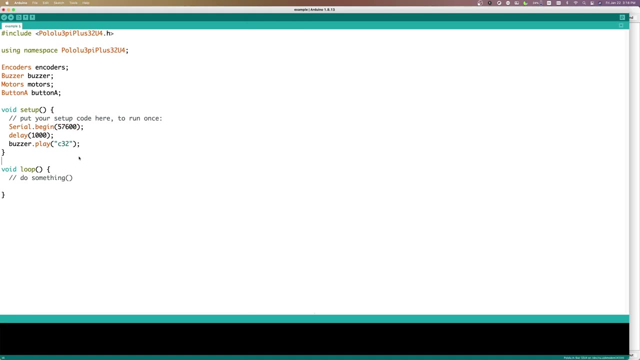 this. you can see that while I'm not pressing the button, they do not show up. But if I press the button, there you go And the robot moves. So success for our first program. Now let's go ahead and bring the wheel encoders into this. We're also going to explore just good robotic and 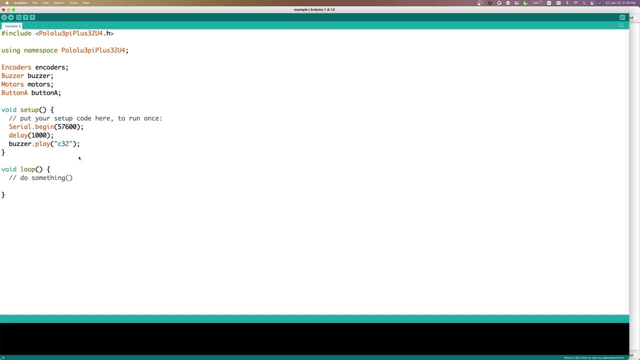 specifically robotic on Arduino programming practices. So one thing I want to address right now is this: So very often you will see loops in Arduino programming where there's some sensors to check or something to do, or LEDs to light up And in order to make that happen, for the time, 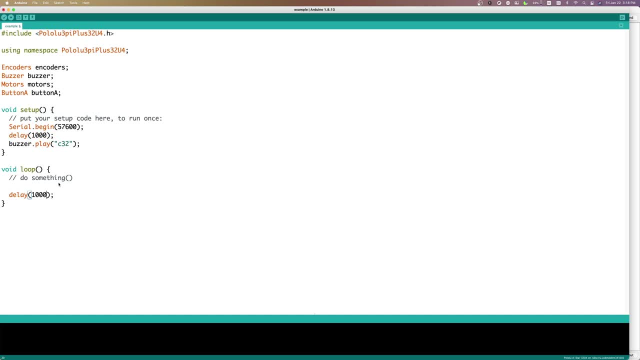 you need it to happen, a delay is added. Now the problem here is that when you get to a delay in this program, it literally sits here and does nothing but run this delay. Any other work that was part of this loop- it's not going to run this delay. It's going to run this delay, So 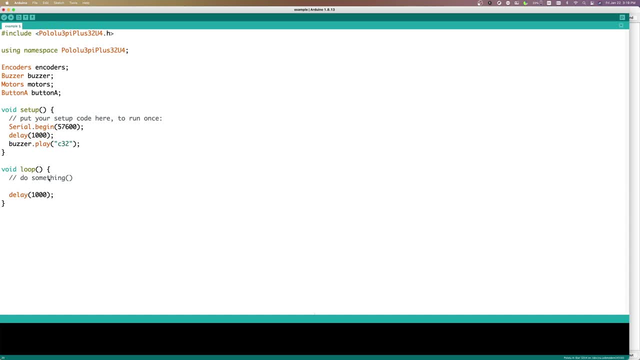 does not happen, whether it's, you know, say, stopping the motors from running or looking at the sensors to avoid crashing into a wall. So we want to avoid that at all costs. What are we going to do instead? Well, the first thing we're going to do is create methods to encapsulate everything. 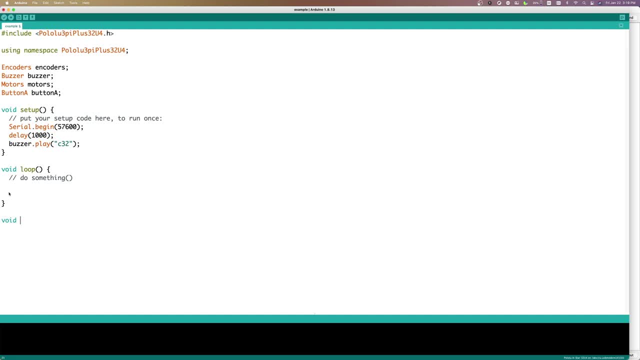 that we're doing Now. this one's a very simple program. We're just looking at the wheel encoders, but obviously this is going to grow over time. So for right now let's just call this check encoders, because we're just going to have this method: check the encoders. It's also going to 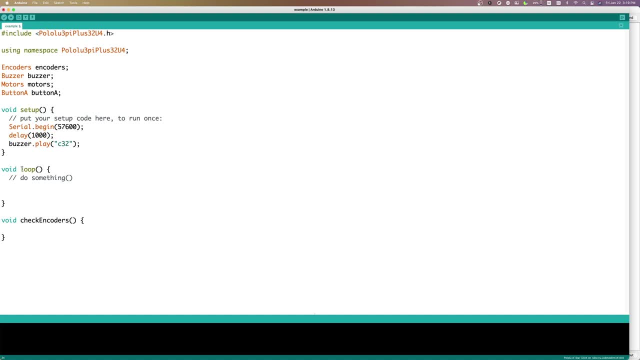 respond to them, but that's fine for now, And we're going to need to call this from our loop, So we'll go ahead and add that as well. Now that we have this, what I want to do here is, instead of worrying about the delays, to separate how often I check my encoders. 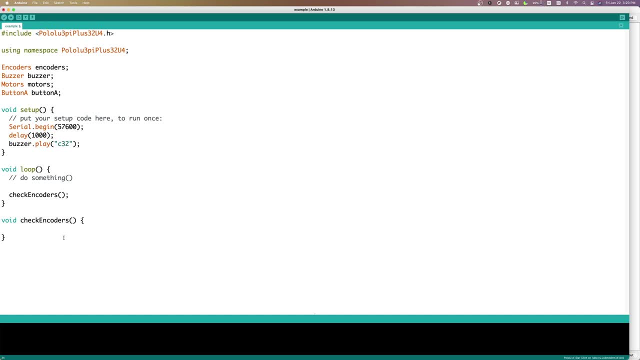 I'm going to use the built-in timers that are in the microcontroller And you can do that very easily by using the millispace check encoder, So you can go ahead and check the encoder and you can see the encoders that are in the loop, And then, if I want to have the encoders in place, I can go. 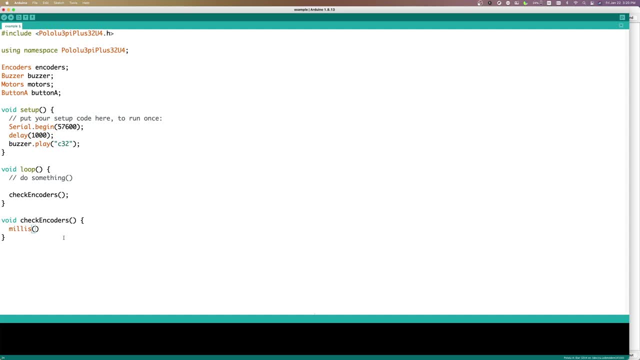 through these encoders to check those timers And then, if I want to have the encoders to check the, the millis function that's provided. The millis function gives you the amount of milliseconds that have elapsed since you turned on the device, So kind of like the epoch time where you know the. 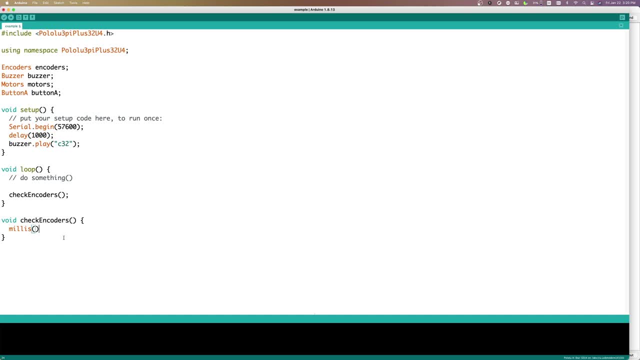 time stamp that we use in computing, where that started on January 1st 1970.. Well, this just starts every time you start the device. Now, to do this effectively, we need to store the information, We need to store the current time. We need to store, say, a previous time that we might have checked. 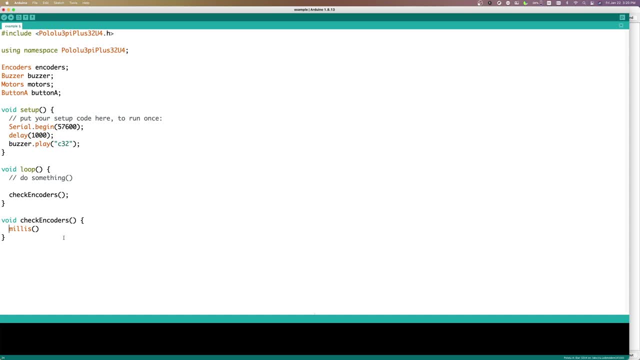 something and we need to know what the interval of time is that we care about that. we want to wait before we check it again. So let me go ahead and create a few global variables here in the global space that we're going to use for that. So the first couple are going to be unsigned longs and 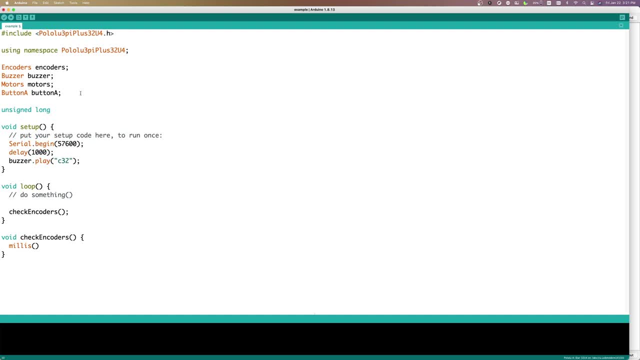 these are going to represent both the current time and the interval of time that we need to store, the current time. So let's go ahead and create a, so we'll say current millis and also the previous time that we'd say checked for this thing. Now, 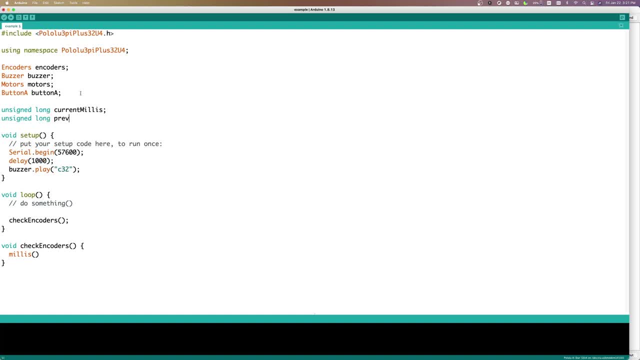 you might have many of these in your program as your program evolves, because you might have ones for checking the encoders and ones for checking the ultrasonic, and ones for how often you check the speed of the motors, So you'll probably end up with multiple versions. 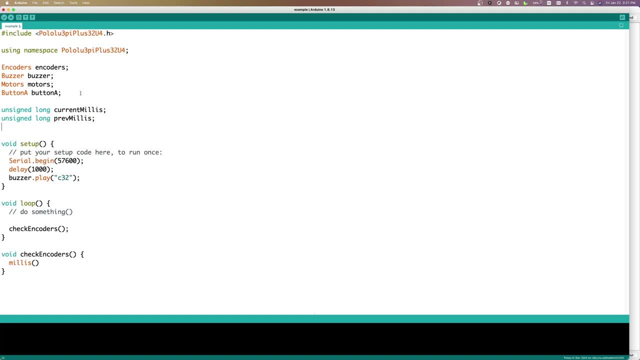 of these and they'll probably incorporate the names of what they're checking. Since we're only checking the encoders here, I'm just sticking with current millis and previous millis, but you might adapt that in the future The last one here is going to be a constant. 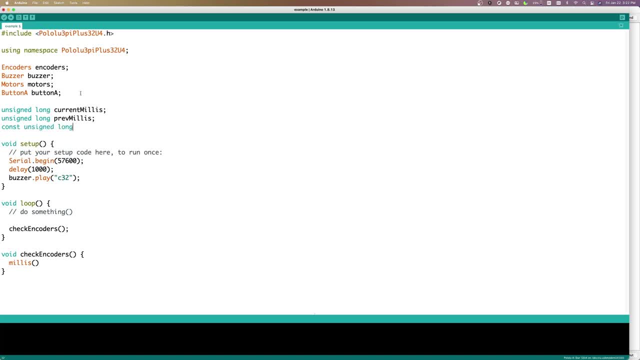 because we're not planning on changing it at runtime at all, and we're going to call this one the period because it's going to represent the amount of time that we're looking to wait before we do this again. I'm going to start off with 50 milliseconds here. Now we might have to adjust. 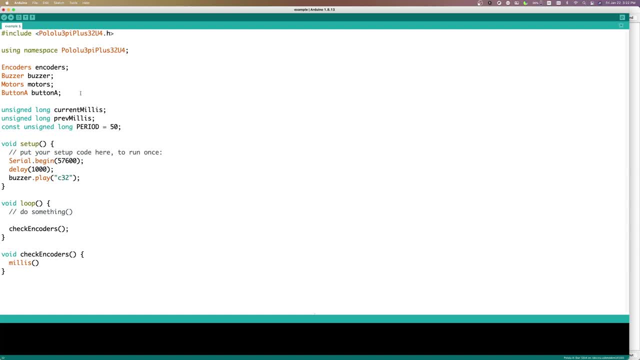 this One of the most interesting parts of programming and programming is that you can see that you're dealing with the physical world and if I say, let's say, I make this 500 right, so every half second I check the encoders. The problem with that is that if I want to go 12 inches, 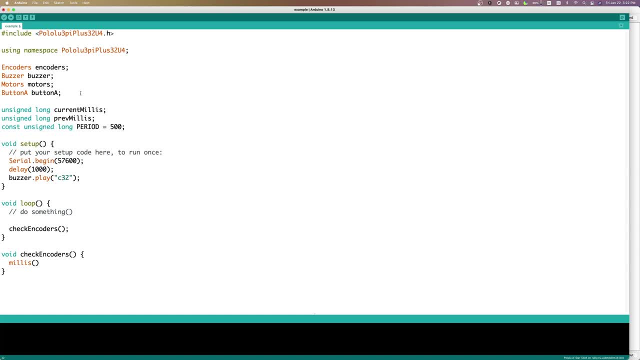 I could very well overshoot my 12 inches by a pretty significant margin, because I'm not checking the encoders often enough to know that I actually went the 12 inches. However, I could make this too small a number. I could say, well, why not check it every millisecond? 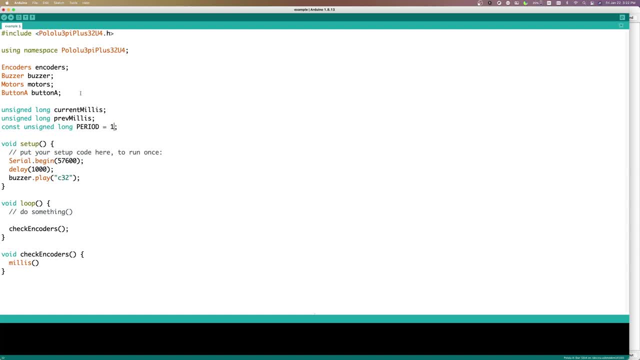 And then my code to check the encoders is running far more often than it needs to and it's taking up the valuable time of the processor from other things that might need to run. There's always a balancing act in doing this, and a lot of it you learn with experience for different types of 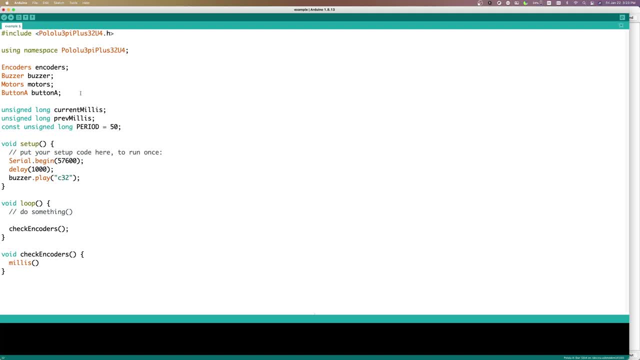 hardware, and a lot of it comes from thinking through the requirements and the probable issues that you could run into. Tuning a robot in the physical space is one of the greatest challenges of programming. If you're a robot and you're a robot and you're a robot and you're. 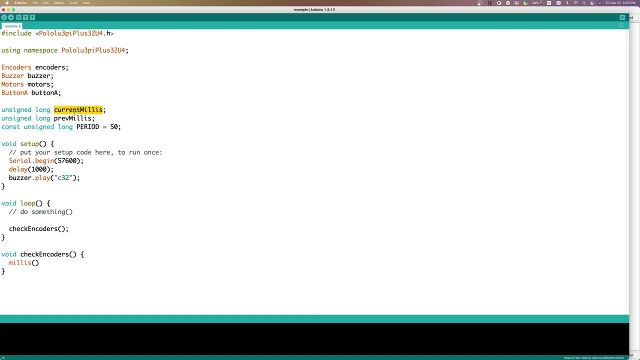 doing robotics programming. So now that we have these, we're going to take our current millis here and we're going to set that equal to the millis that's recorded. So we're going to do that every cycle, which this is going to happen as fast as the loop can get through all our code. So this is 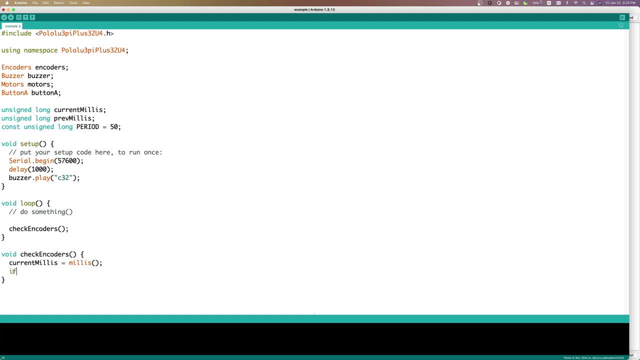 going to happen quite often, and now we're going to use that information to check to see: is the current millis greater than the previous millis plus the period that we mentioned before? right has enough time elapsed in combination with when we last ran this to run it again, and we will only go into this block every 50 milliseconds or longer. 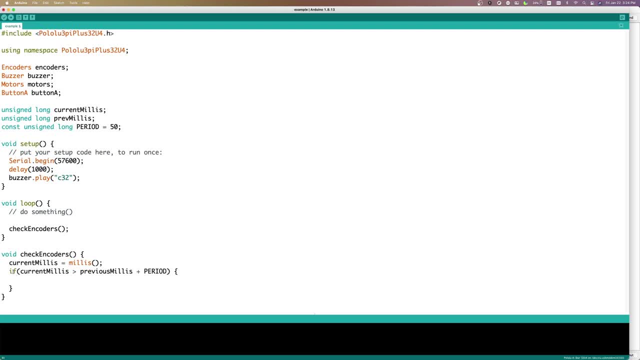 because, remember, depending on what else is going on, there's no guarantee that we're going to check this exactly at 50 milliseconds. If some other function was running that took a lot of CPU time and the 50 milliseconds elapsed, then we're going to run it again. So we're going to run it again. 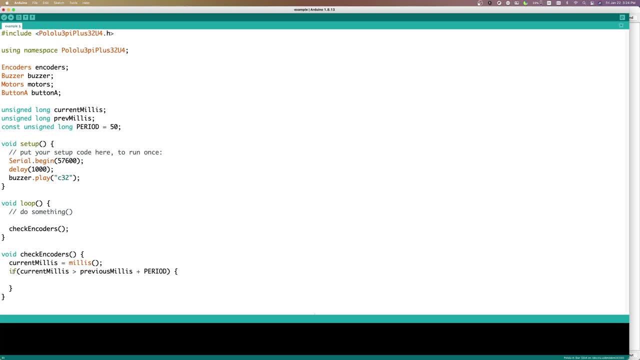 and say we went to 60 milliseconds. well, this will still be valid and we will still run this code, albeit 10 milliseconds after the minimum amount of time that has to pass. Also, keep in mind that we have to, as part of this, set the previous milliseconds, so it's good to kind of do that now. 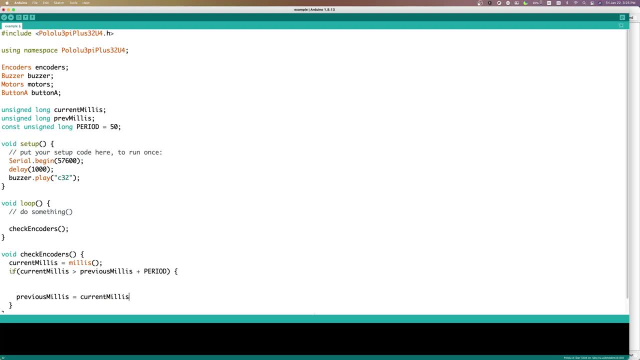 just before I forget. So I'm going to set that equal to the current millis at the end, and you want to do that at the end of this block. So now that we have that that up, we can actually use this code to do some checks. 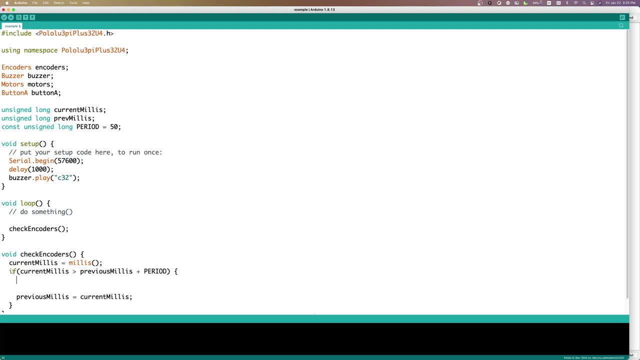 and to look at the encoders. So let's do that. The first part of looking at the encoders is again going to be setting up a couple of variables. Now I'm going to actually set these up globally, but they don't need to be, especially in this example. 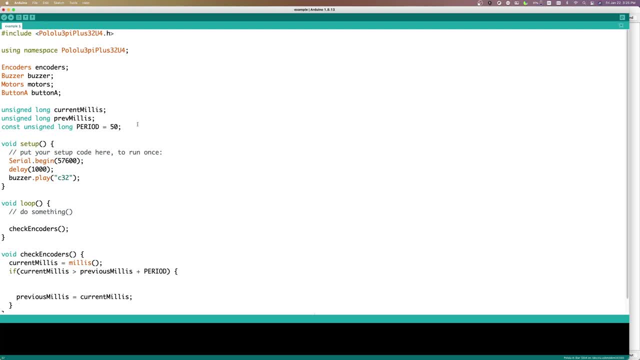 I can actually run all this code right within this method, but commonly in these kinds of things you're going to be using the results of this in other places, say in a function that deals with using the motors, maybe in some of your other functions. 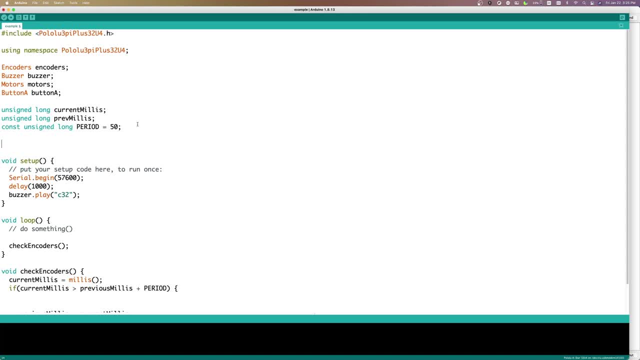 that deal with the actual mathematics localizing the robot, going to create one called counts left- this is going to be the variable that we're going to put that into for the left wheel and counts right for the right wheel, And I'm also going to use again a previous counts. 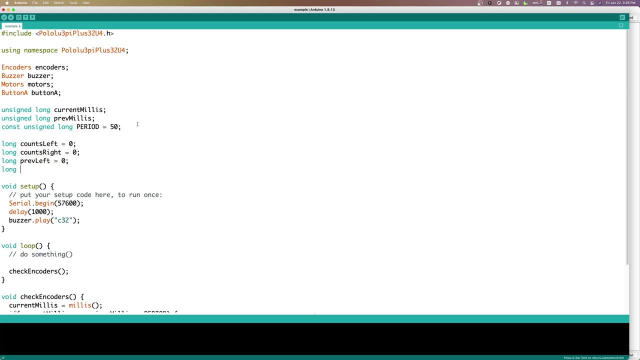 So I'm going to say previous left and previous left And I'm also going to say previous right as well. Now that we have those, we can come down here and we can assign them And remember- I don't want to reassign- 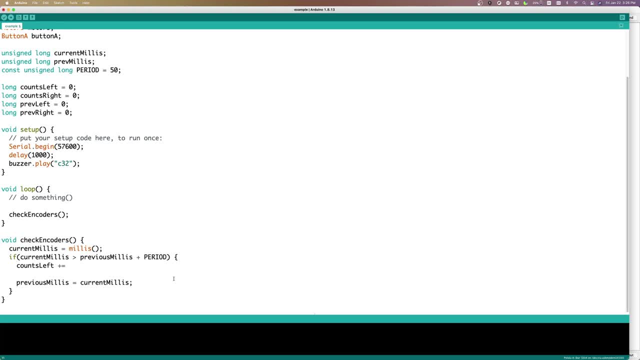 I want to add on every time right. So if I get an encoder count and one iteration of this 50 milliseconds or more later when I come to the second iteration, I don't want to overwrite this. This is the total count I want to add to it. 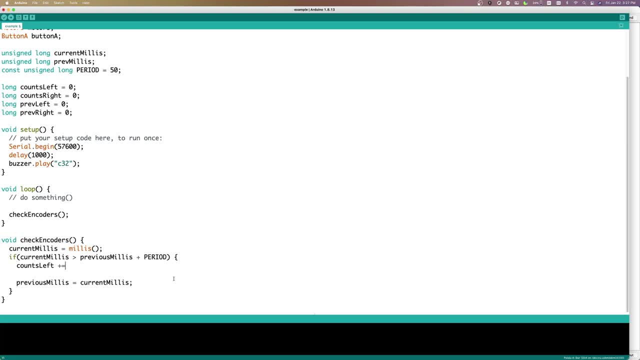 So this is the equivalent. we say plus equal. This is the equivalent of saying counts left equals, counts left plus, whatever I'm going to add to it. And what I'm going to add to it is the value I get from the encoders. 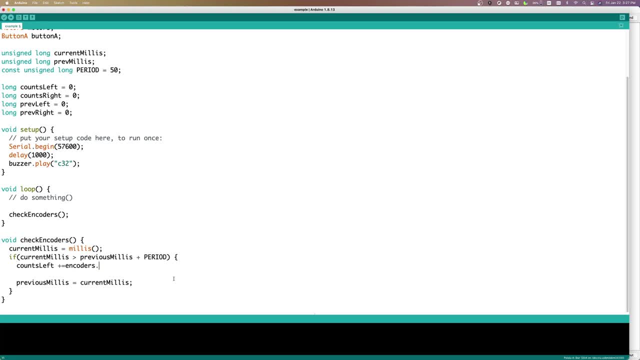 So we say encoders dot. the method I actually want to use is get counts and reset left. Now, the reason why I want to do this is there's only a limit. I believe it's 32K or 32,000 on the register. 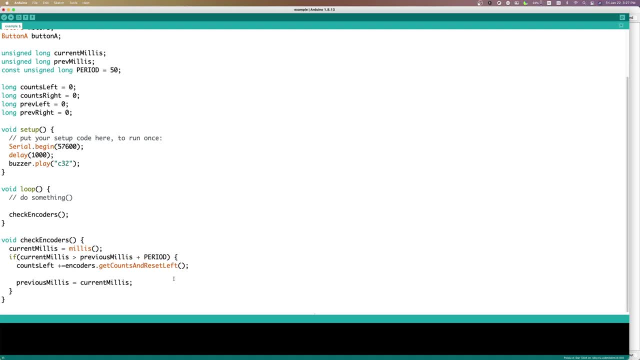 that keeps track of the encoder. As it goes, that actually overflows pretty quick. So in a turtle that has a 75 to one gear ratio, I want to say it's like 30 seconds, depending on the speed of the motor of course. 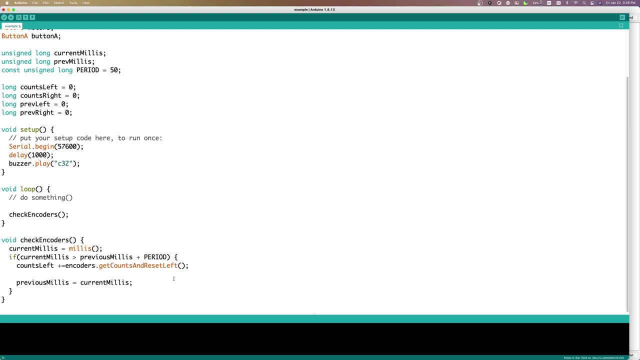 but it's not very long. You're going to want to reset this often and you're keeping track of the count and you're longer, long, right, So there's no reason to really not reset it often. So every time I retrieve the value. 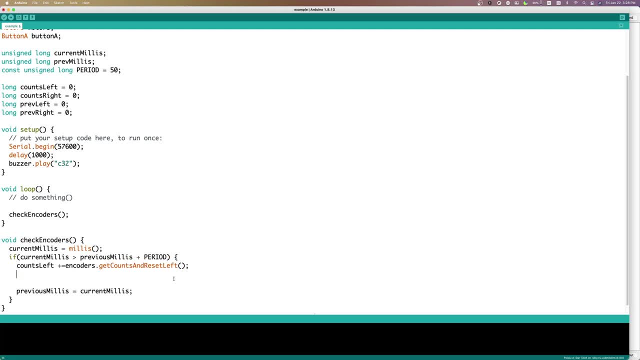 I reset the register so that I'm less worried about it Overflowing in the future. I'm going to repeat this for counts right. And now that we have that information, why don't we just simply print it out? So we're going to do serial print. 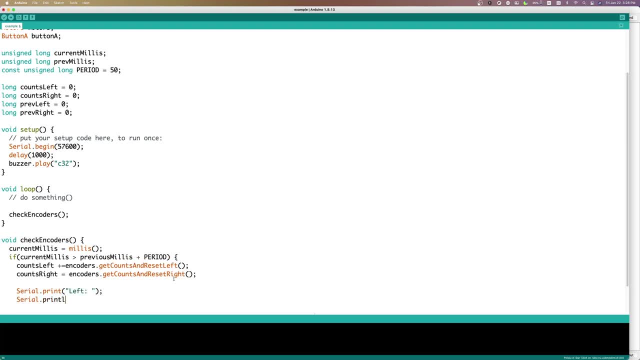 and we're going to do laugh. Let's do another serial print here. We're going to have the counts, laugh, And what more here. Now I mentioned earlier, concatenation doesn't really work in this, So this is how you effectively do that. 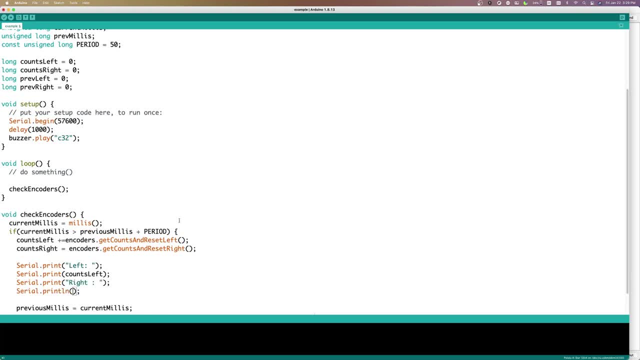 And then, in the last line, we go ahead and put our println Now also want to space there. It'll look funky, And here is our counts rate. Okay, So let's see if this compiles. Let's see how the demo gods feel about me. 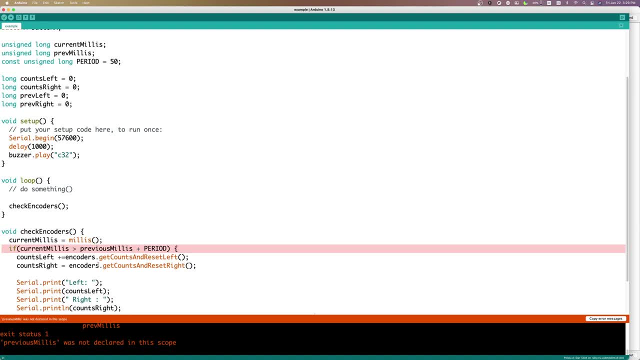 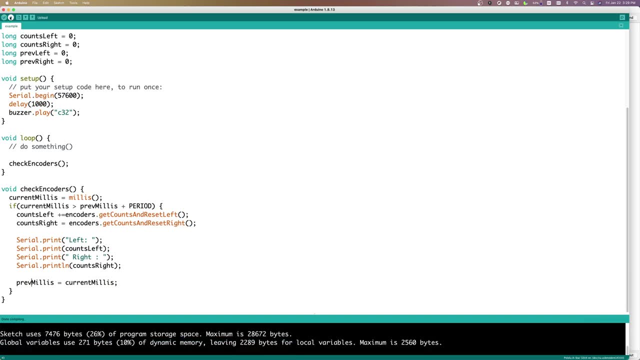 Previous millis not declared. I called it priv. that's why. So let's take the IOUs out. Same thing And let's try again. All right, looks like we're going to go that time And we did, All right. 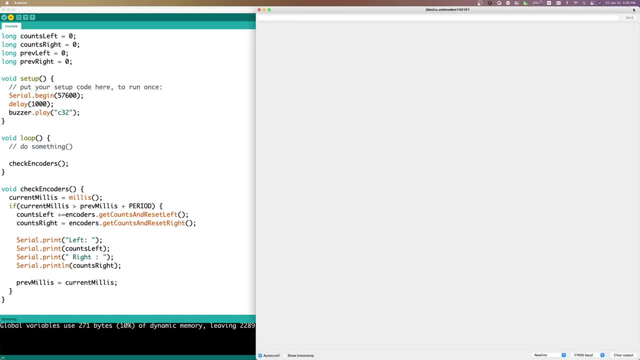 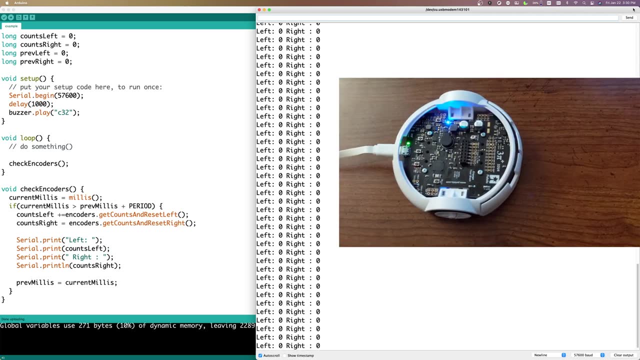 So we're going to compile and run. Let's open our serial monitor here And there you go. You can see our left and right coming up as zeros. Now, of course, I haven't applied any motors. I took that code out. 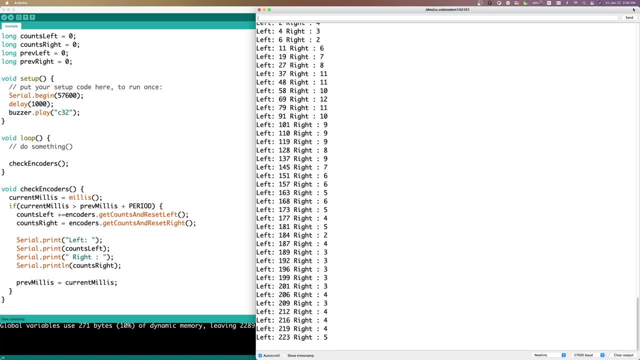 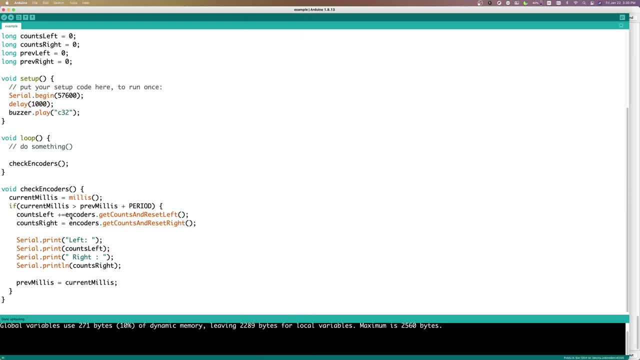 So I'm going to physically move the robot and you can see that they are. in fact, one of them is going up and notice, the other isn't. because, after giving that whole speech about adding, you know, continually and not replacing, I didn't do it for the right one. 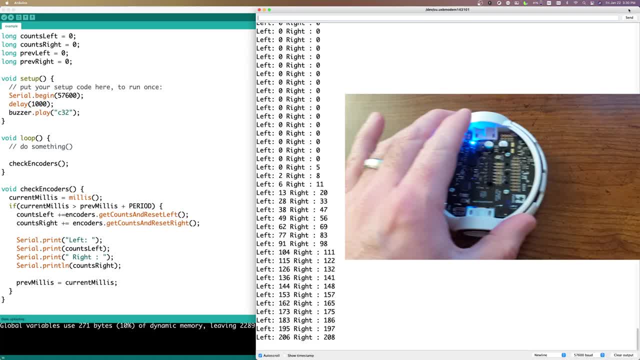 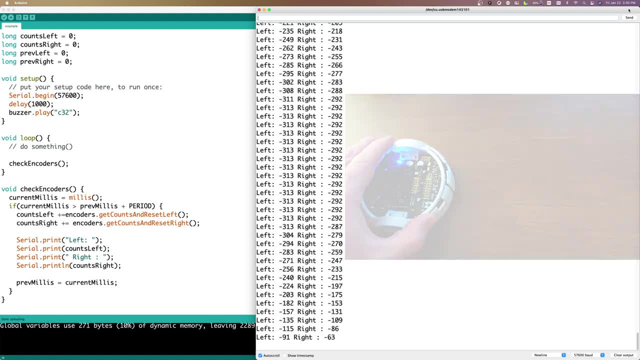 So let's reset that and do it again. And there you go. That's much better, All right. So I'm just moving it back and forth. You can see if I move it back further that I go into negatives, And if I move it forward I stay in positive. 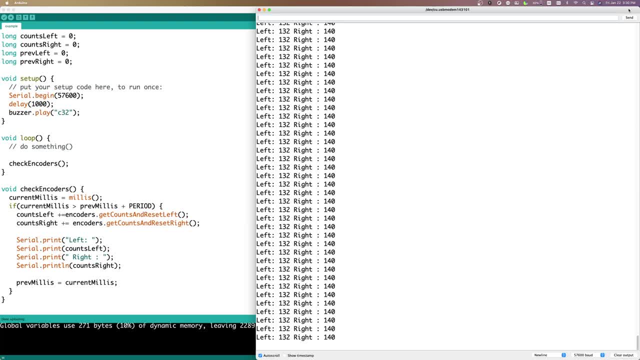 So that's great. So we've accomplished one goal. We've accomplished reading the encoders and being able to display that out. And just to play around a little bit here, let's change the period So we can kind of get a feel for how fast that is. 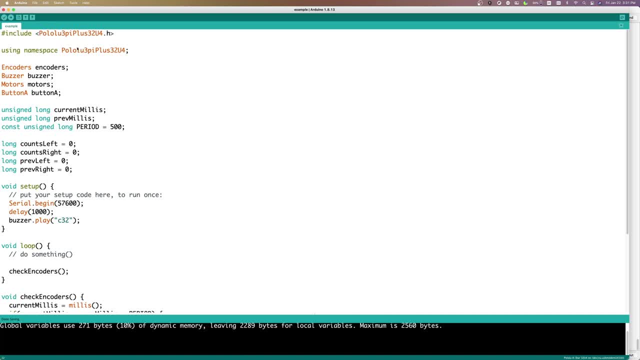 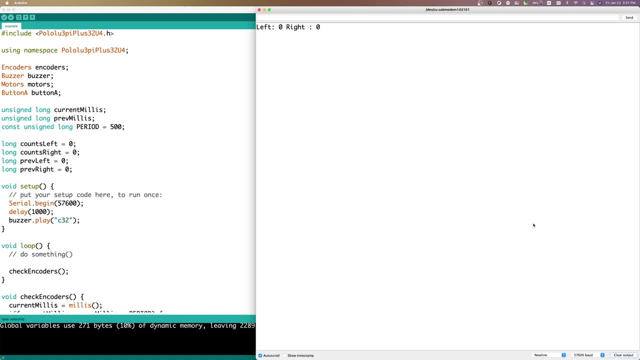 Let's change it to 500, just so you can see the difference, And we'll upload that. come back over here And let's clear this, just so we can see it fresh. And now you see every half second it's updating. 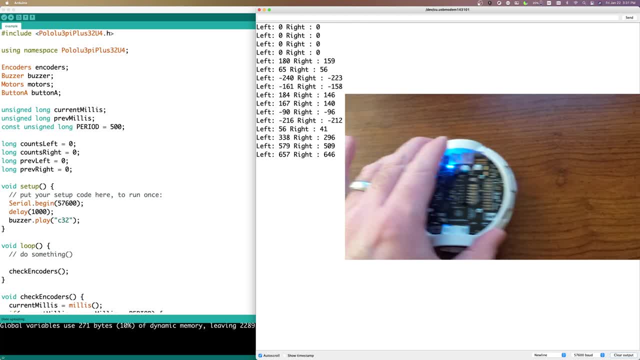 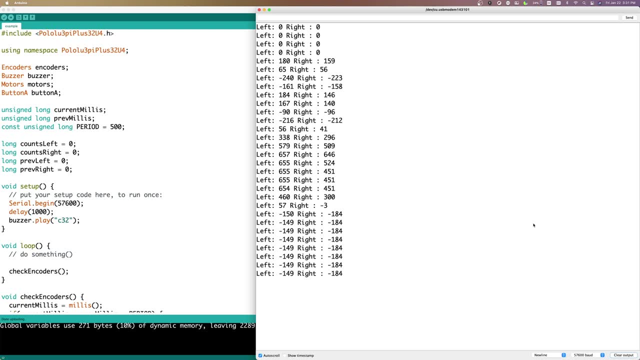 And look at how much of a lag that is. I mean, if you imagine that I had gone past a certain distance, you can see that quite a bunch of clicks happen in between, And I mean I'm not even pushing this thing very far, very fast. 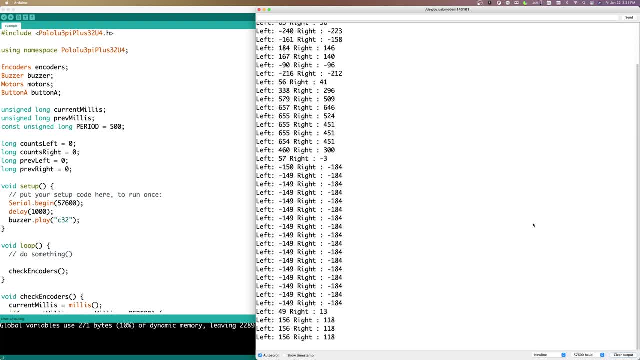 And this is a standard edition, not the Turtle. The Turtle numbers would be more than twice as fast as these because of the gear ratios. Just something to keep in mind. Again, that period is very important. I'm going to put it back to 50 milliseconds. 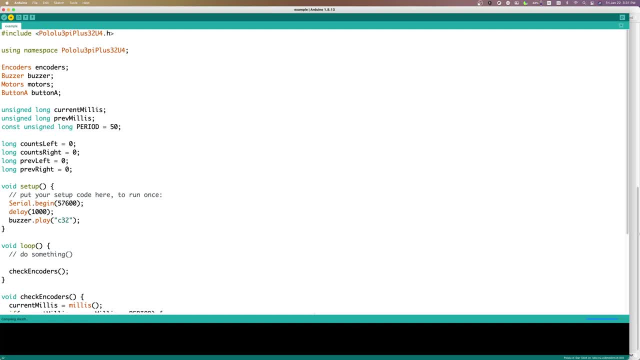 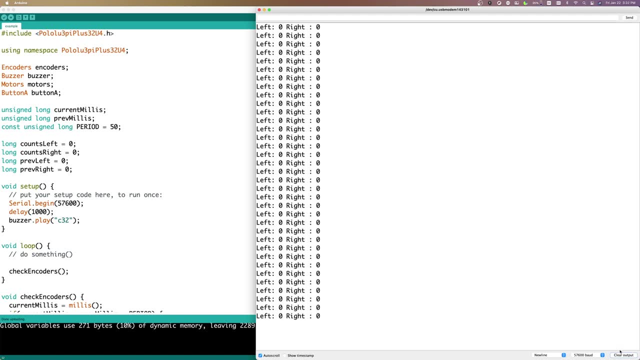 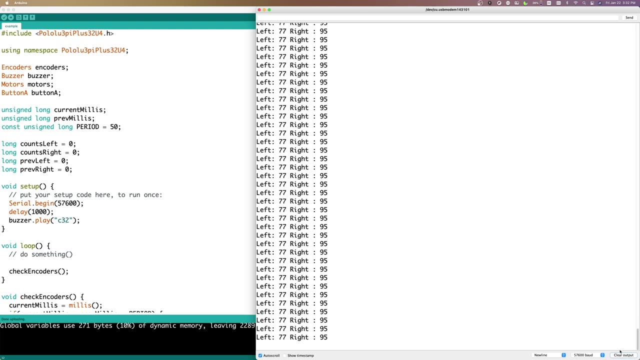 Let's reset that, Reset this to clear it And again you'll see the difference right away, because this is going to scroll right off pretty quickly. Now that we have the encoder, let's learn the math that we need to actually convert that into distance. 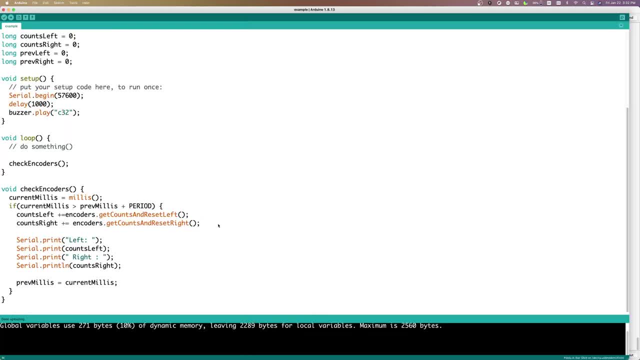 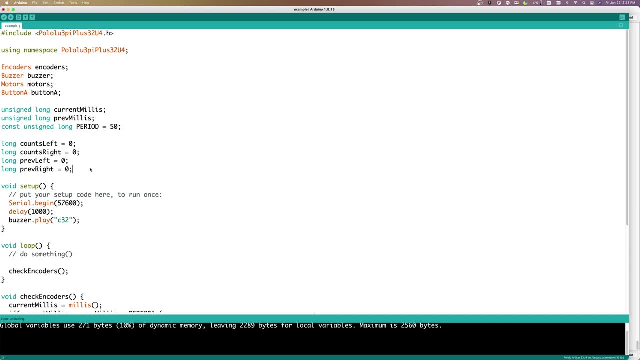 We're going to convert it into distance in centimeters. So to convert it into distance, we're going to need distance in centimeters. We're going to need first two variables, which I want to be floats because these could be fractional numbers. 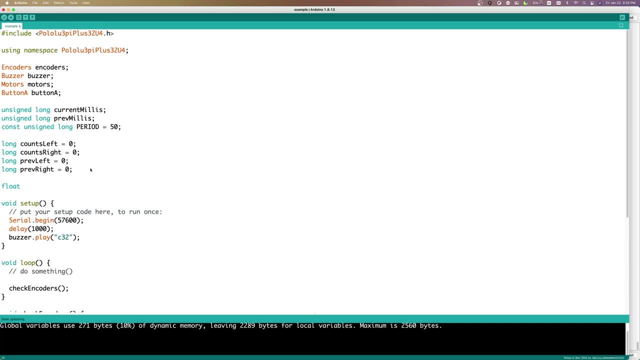 So we're going to call them SL for the distance traveled by the left wheel and SR for the distance traveled by the right wheel. So now that we have our SL and SR to keep track of wheel rotation, let's add a few more constants that we're going to need here. 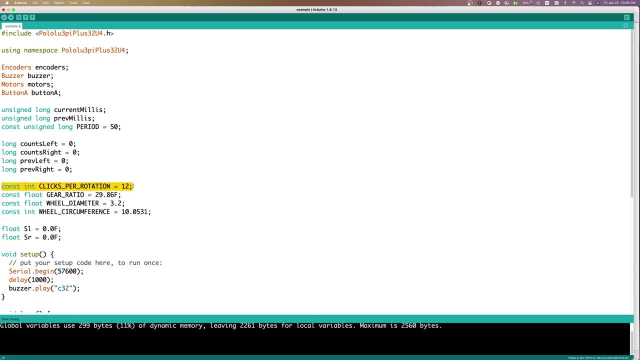 I'm pasting these in and I'm going to go through each one, one at a time. So the first one here is clicks per rotation. Now, this is specifically referring to the rotation of the DC motor and the encoder shaft. This is every single time the DC motor makes one full rotation. 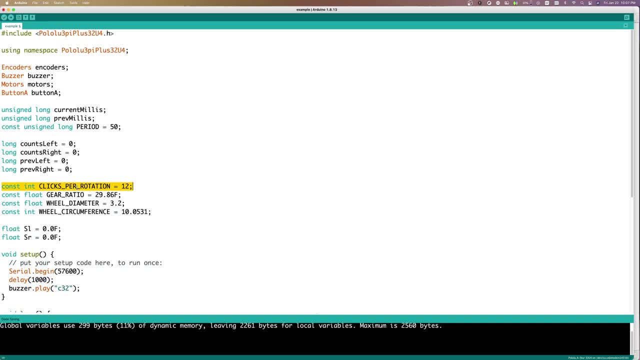 there are 12 state changes acknowledged by our encoders. Now, that is not the clicks per rotation of our wheel. Remember that our DC motors have a gear mechanism to actually slow down the DC motor's rotation and increase the torque. The standard edition that I'm using is a 30 to 1 gear ratio. 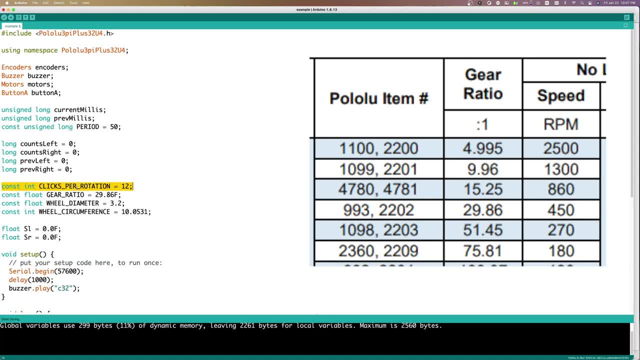 Now the very specific. as shown on the data sheet here, gear ratio is actually 29.86.. If you have the Turtle Edition, this is actually, I believe, 75 point something. And the Hyper Edition is even slower than this one. 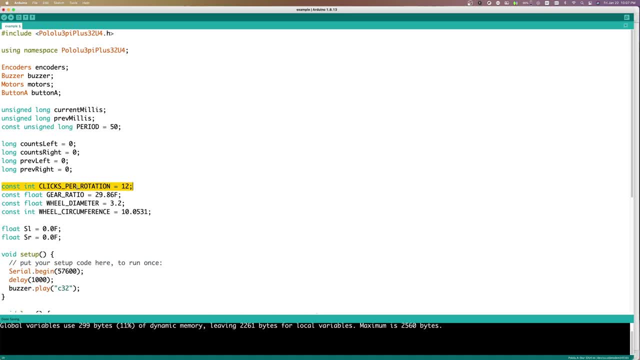 at 15 point, something That means that the Turtle Edition actually shows the most clicks because you've slowed down the wheel and increased the number of clicks that happen at the shaft of the DC motor before the wheel fully rotates. The slower the robot goes, the more clicks. 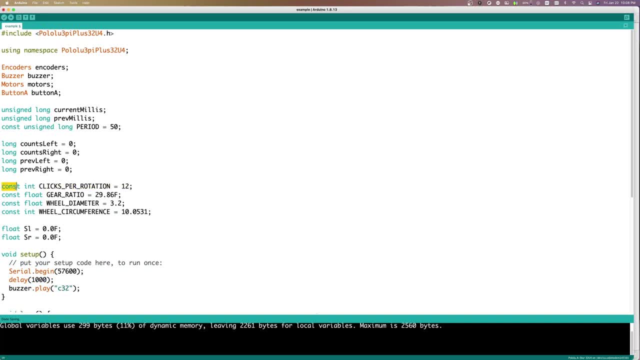 you get per rotation The combination of these two things. when we multiply them out, give us the total number of clicks that happen for the encoder per wheel rotation. The next thing we need to know is the diameter of our wheel and the circumference of our wheel. 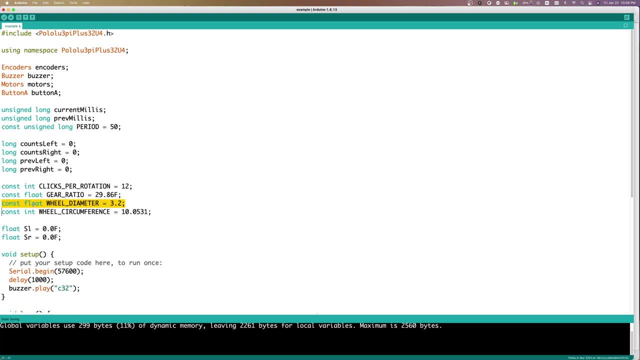 Now we know that the circumference of our wheel is the diameter of our wheel, times pi. The diameter of our wheel we can luckily look up, as seen here, using the Pololu documentation. So it's a 32 millimeter wheel. 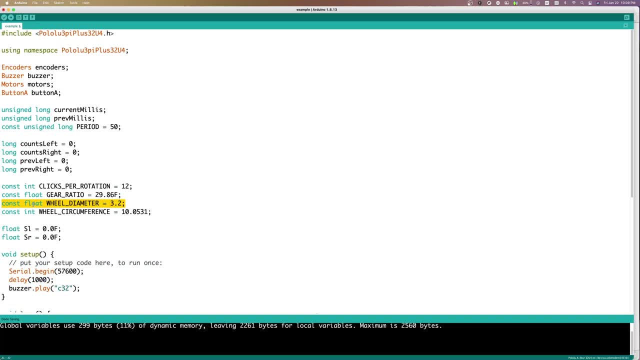 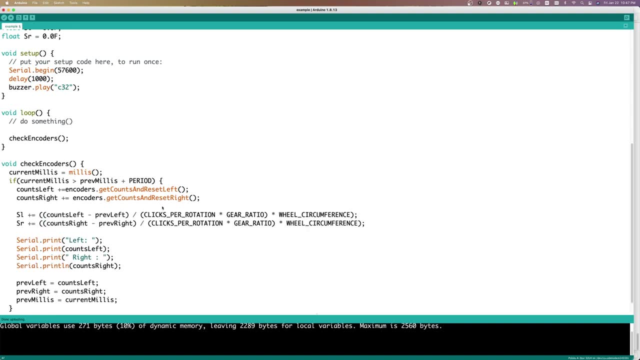 We are going to be using centimeters, So once we have our wheel diameter, we can figure out our wheel circumference. So now that everything is set up correctly, let's paste in the equations that we'll be using here And disseminate what's going on. 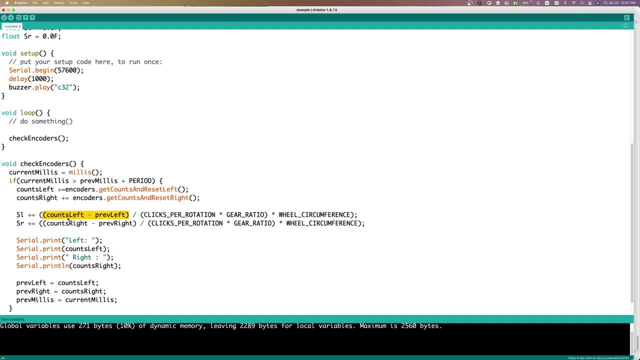 I want to start with interparens first. So the first thing I want to note here is that we're getting the difference of the counts. So remember just the difference that happens each time we come and pass this period and check. We're going to be dividing that by what happens in here. 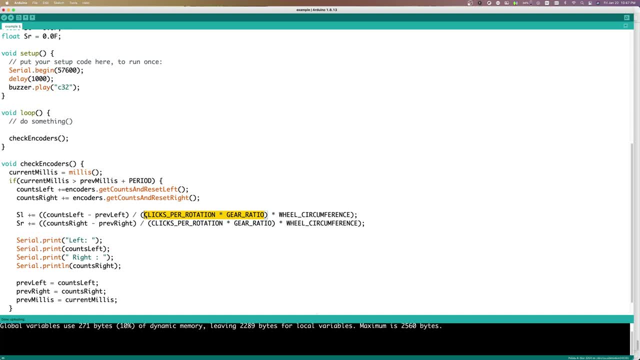 This, remember, is the clicks per rotation of the actual DC motor times the ratio of the gears giving us the rotation, or the clicks per one, One rotation of the entire wheel. We're then going to multiply that by the wheel circumference. The total result of this is divided. 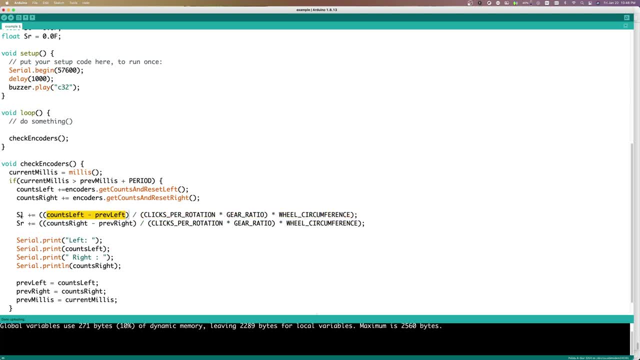 by the actual number of clicks, which gives us the distance achieved in that number of clicks. That's what you're going to find in here in centimeters. This is obviously the same exact thing for the right hand side. Let's go ahead and change these values out here. 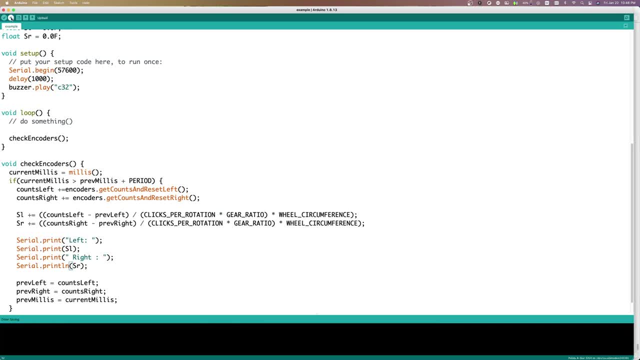 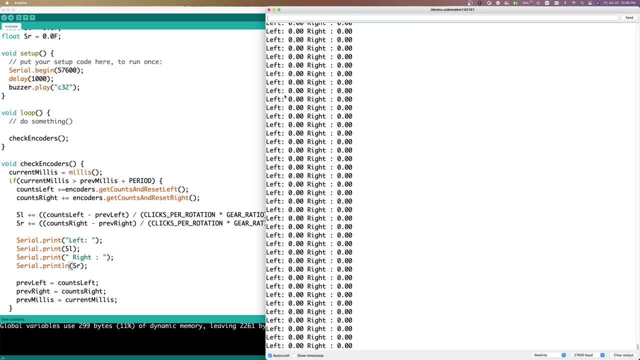 so we can see what we're looking at. Let's do a compile and a load And let's go to here And you can see here that we now have left and right with floats And let's see what happens when we move them. 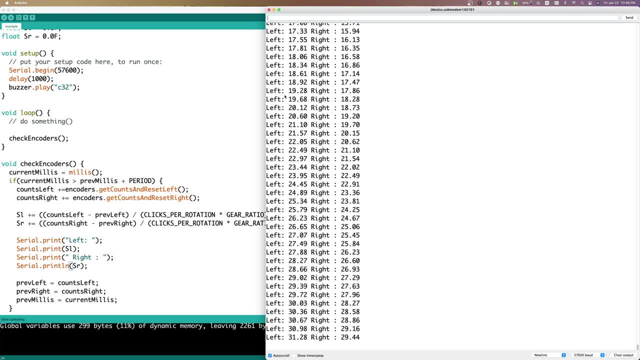 Look at that. Now we actually see the centimeters And I'm going to move it. I went over about 12 inches And that is about 30.5 centimeters, And that is how far we're going to now tell the motors. 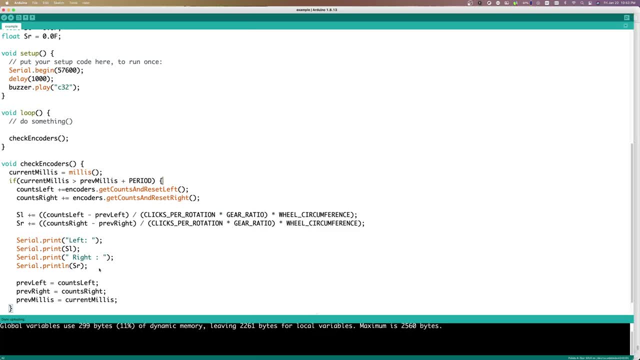 to move it in the very next section. So this is very good And we have it measuring distance- But we just need to use the motors to now try to go a certain amount of distance. Let's give ourselves some space here and take a look at the code we're going. 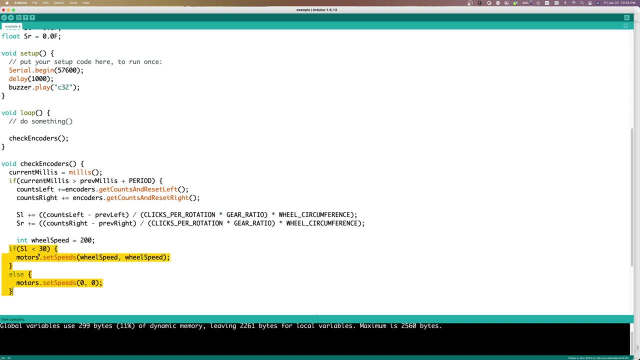 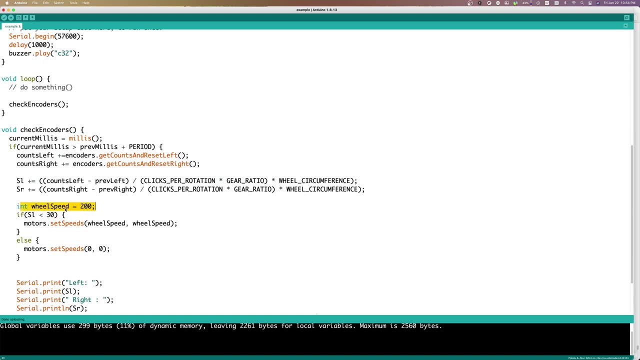 to be bringing in in this section. So what I've done here is essentially just create a integer variable to contain the wheel speed, which I've set at 200.. I could have just written 200 here. However, I might want to change it. 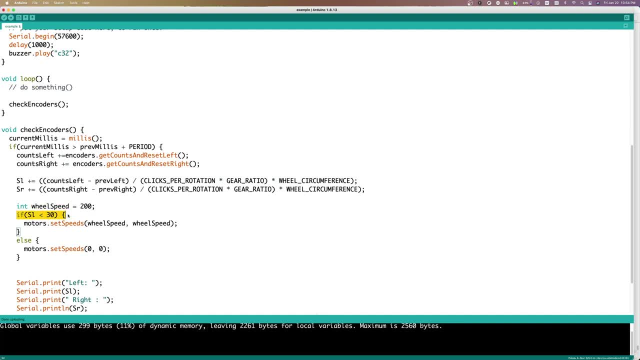 So this made my life a little bit easier, And this is important. Notice here what I'm doing. I'm saying: if SL is less than 30, I'm going to set the motor speed to what I said here, And otherwise I'm going to stop. 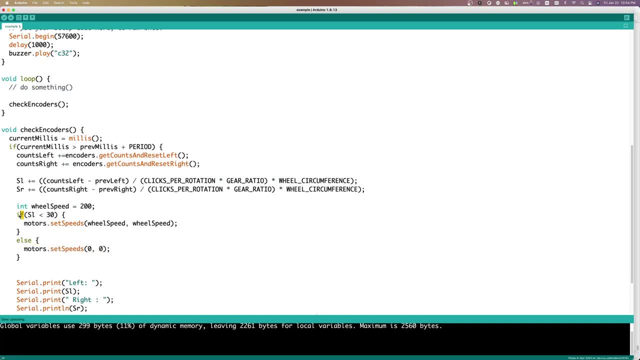 Well, that seems pretty straightforward, And it's correct for what we're doing here in Arduino, But I want to point this out because most people would probably be inclined to do a while loop here or some kind of for some looping mechanism. We have to consider, though, what would have to happen though. 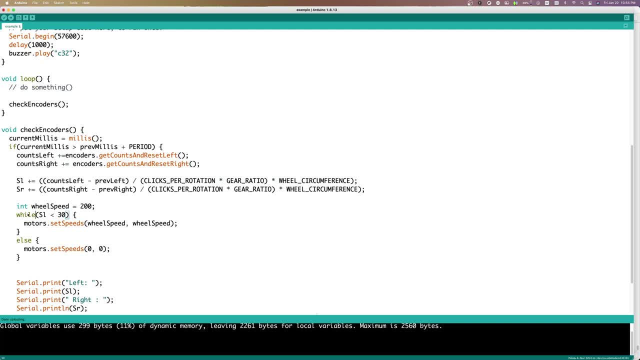 what would happen if we had done that? Remember, if we're in a while loop here, this SL value is not going to get updated because we're never running this code while we sit in this loop. So this breaks what we want to achieve. 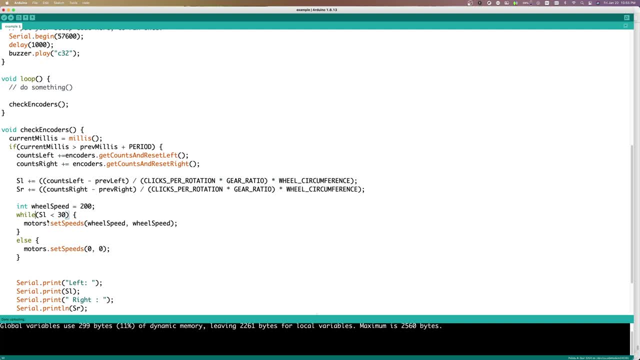 And this is a very common problem when you're dealing with microcontrollers and, in particular, Arduinos. Remember you are in a loop. If you find yourself wanting to create a loop, consider instead what is the condition that I would check in this loop? 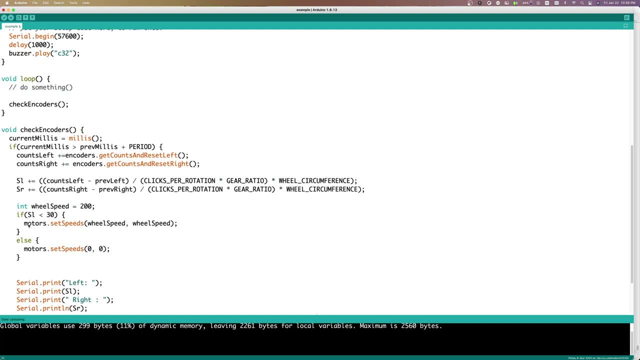 And can I instead just use an if statement and the existing loop that I'm already utilizing as the looping mechanism? So here I am, simply implementing that condition to say, wow, this SL is less than 30.. Let's go forward, Otherwise we're going to sit still. 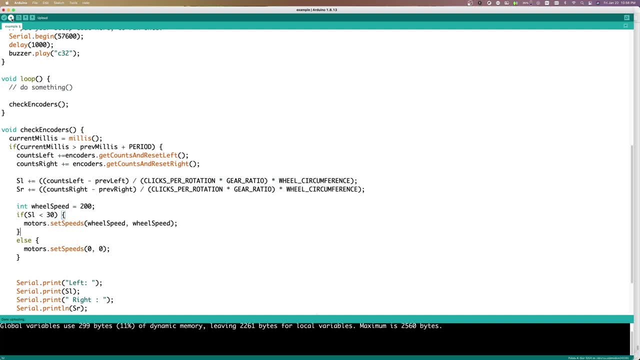 Let's go ahead and see how this runs Now. be aware, when you do this, your robot is going to be moving And if you have a bug or something, maybe more than you expect. So hopefully it's a foot, But just be aware and ready to catch it when it starts moving. 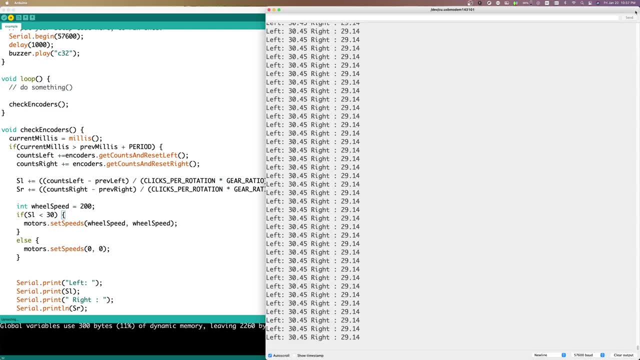 Let's hit upload And we'll see our speeds here. Clear the output And make sure to turn your motors on. And boom, it went and it stopped. I'm going to do it again here. Let's clear our output and run it one more time. 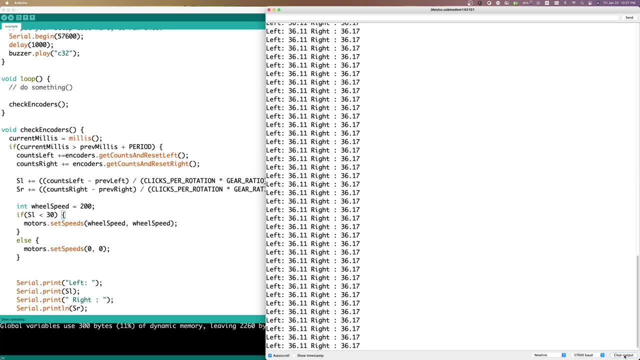 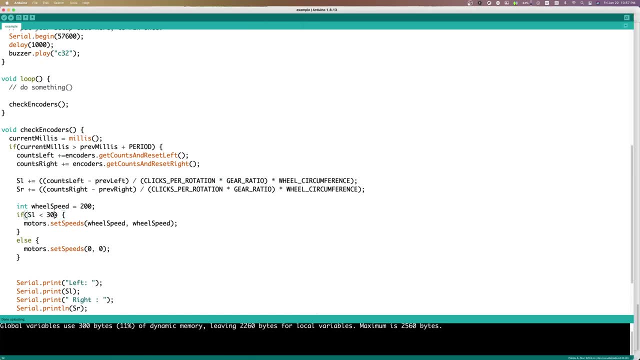 And there you go. Now notice that we are getting a little bit more than the 30 we expected. In fact, I do want to point out here that I said it was precisely 30.5, and we didn't actually do that. 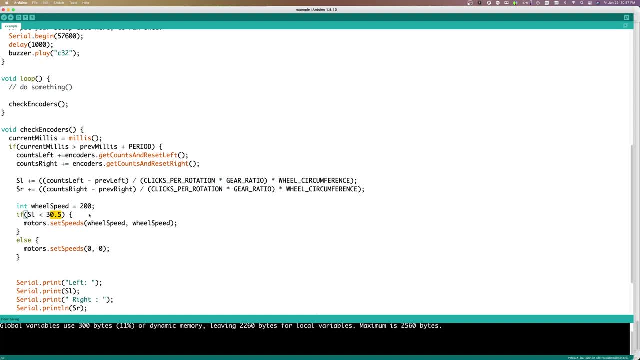 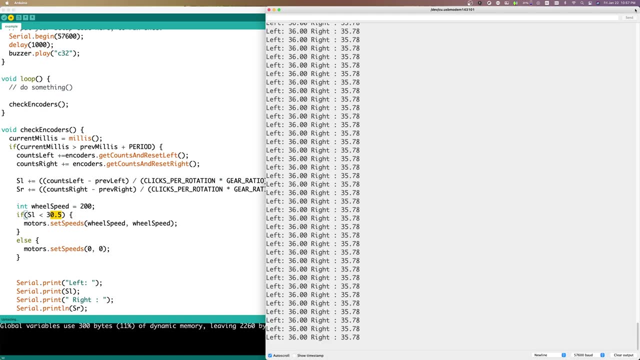 So let's be more precise, shall we? But that's not going to fix our problem, In fact. let's just go ahead and upload this and see what happens when I do, And the answer is that we still got even a little bit further. 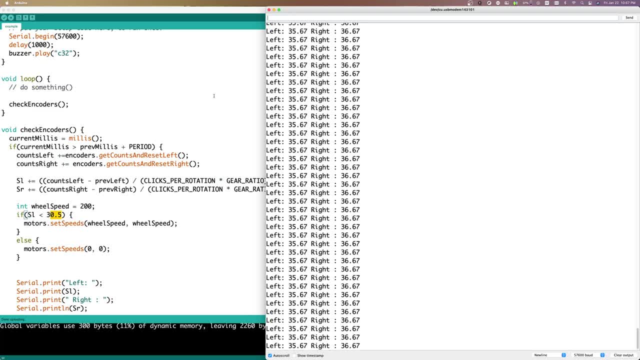 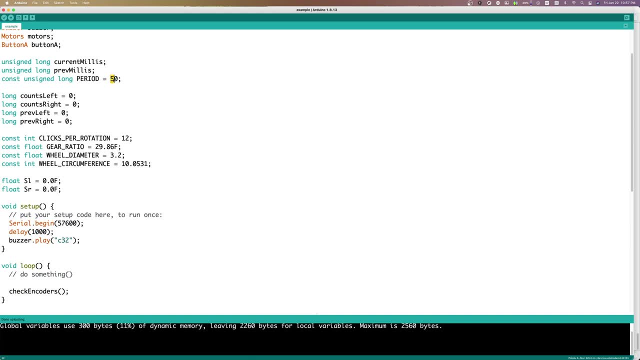 than we thought Now. if you remember, when we discussed the amount, the amount of time that we had here in our period, we said that something like this might happen, that we might not check our code often enough in order to respond quickly. 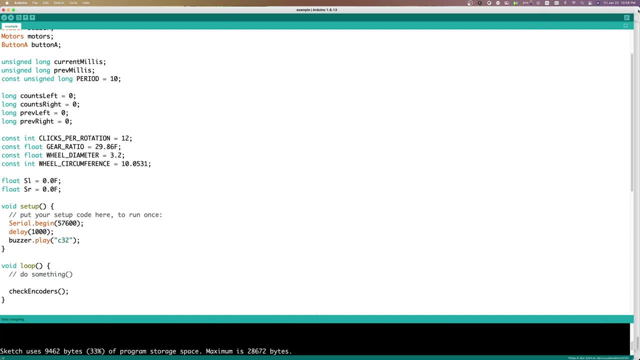 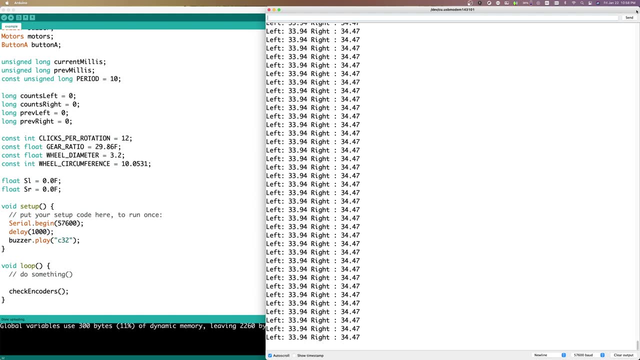 Let's see what happens if we drop it down to 10.. That was pretty consistently reading the 35, 36 range. Let's see what happens now. Oh, better- Not perfect, but better. So this is a great example of things. 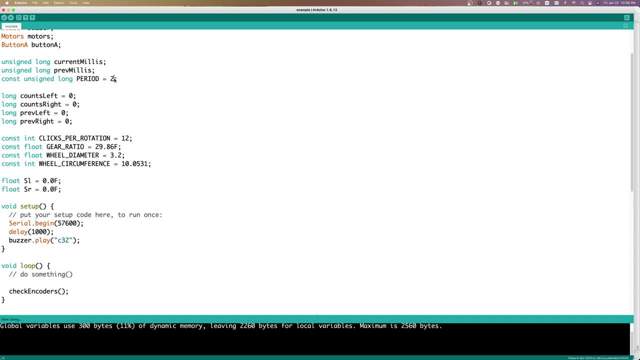 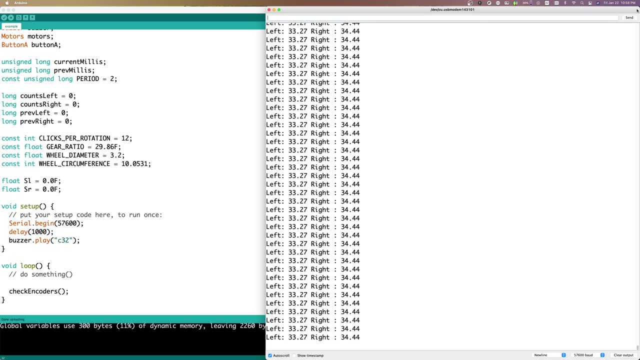 you have to watch out for, Just out of curiosity, let's take this all the way down to a period of two and run it one more time. So we definitely had a better result that time, And there it's about as good as we're going to get. 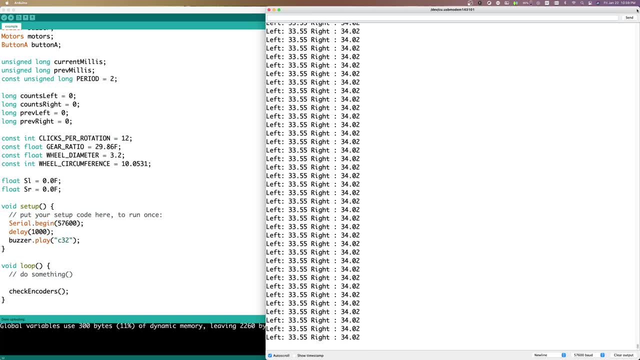 Now I know another reason why this is failing, and it actually is not the period, And this is important, because you could struggle with this and say, ah well, what's going to happen now? I can't actually lower the period effectively anymore. 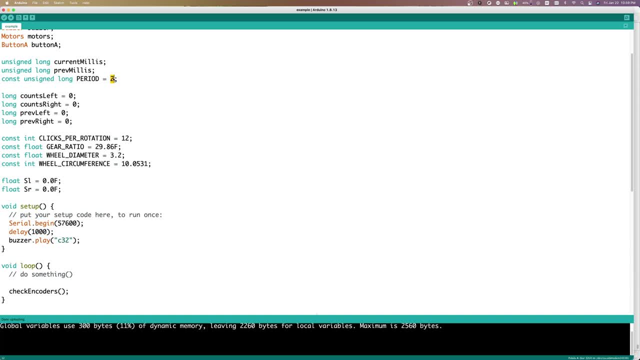 It's not too heavy, It's just a matter of trying to figure out what's going on. So two had no difference from 10. In fact, let's bring this up to 20 and see if it even makes any difference at all. 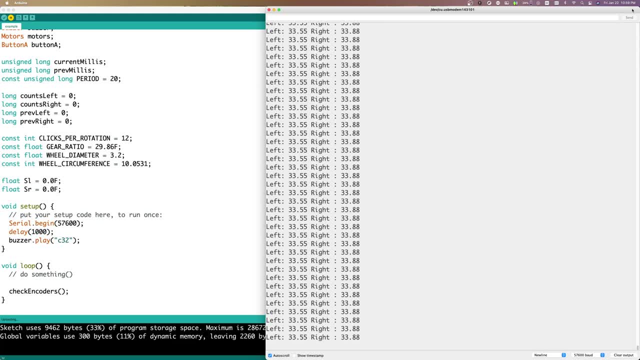 This is a good time to try to figure out tuning-wise what is the period that. I need to be as precise as I do, And the result for 20 is exactly what the result for 10 was, So 20 appears to be a good number. 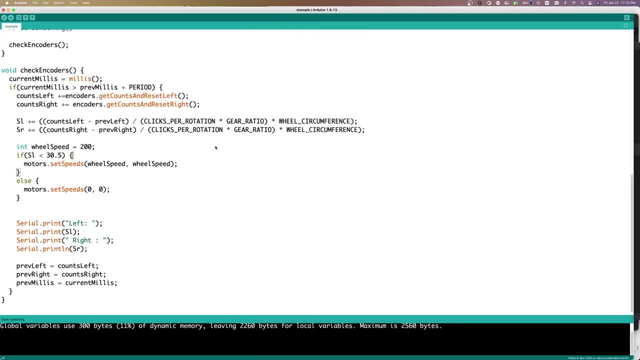 Let's stick with that, But we're definitely further than we want to be. I mentioned earlier that a large portion of this time, that we're going to be doing this in a very short period of time, but we're going to be doing this in a very short period of time. 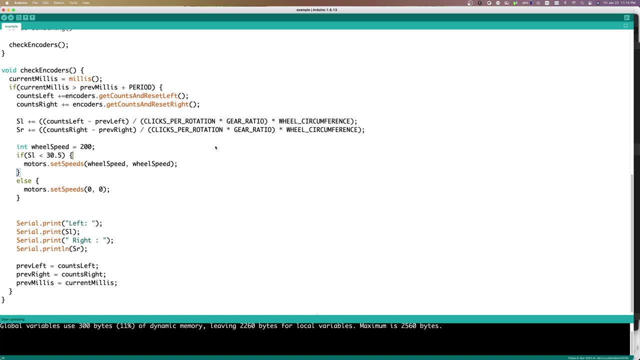 the effort and what makes robot programming unique is tuning it for the real world, And we've now seen that just in looking at how quickly we update mechanisms that read the encoders and how quickly we pull distances from there have a real effect on how precisely we 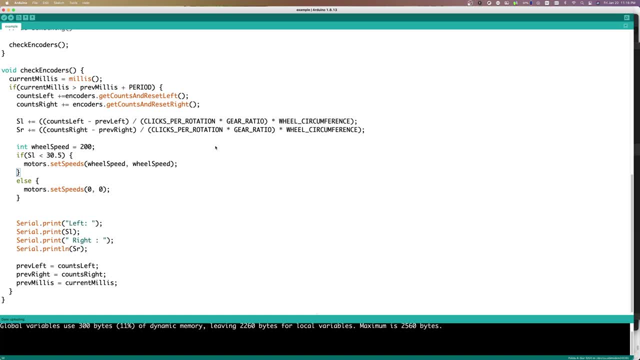 can come to meeting our goal Now, another big thing that's going to have a factor is speed. Now, I guarantee if I lowered this speed right now, right off the bat, it would actually improve our situation, but it's still not going to get us precisely where we need to be. 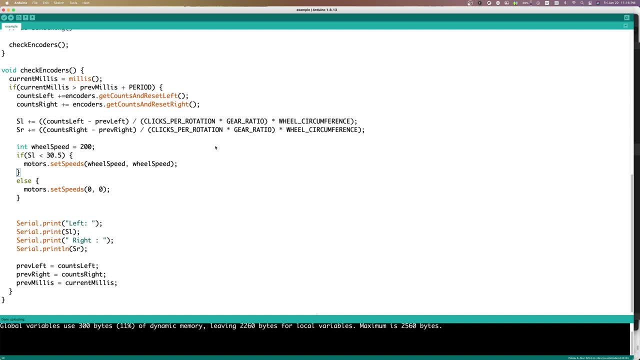 And the reason for that is because you might have noticed my pretty quick standard edition here- moving at half speed actually makes an audible thump when it gets to the end, because the back end is actually flipping up and it's moving. It's moving forward a bit further than it should. 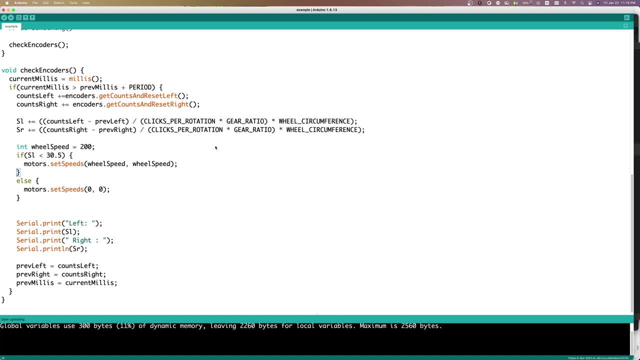 Imagine getting in your car and driving at 60 miles an hour And effectively trying to stop instantly. That's not going to happen. Now, obviously, our robot does not have the physical weight of a car, but it still has to deal with this problem. 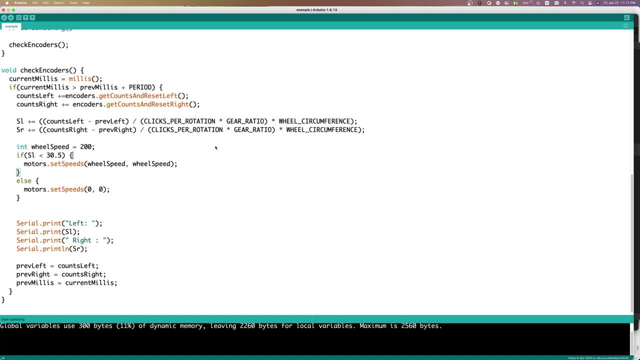 Now, this problem I'm describing- I mentioned earlier- is known as the dynamics of the robot, And we can try to overcome that here, maybe by slowing ourselves down as we approach the finish line. So more to make the math easier and also to make this more controlled, because you 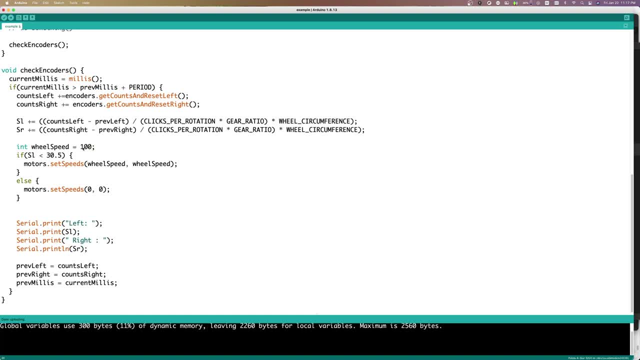 don't just get to go as fast as you want for free. If you want precision, you might have to slow things down. I'm first going to slow the robot down, but that alone isn't going to be enough. What I'm then gonna do is add this code here: 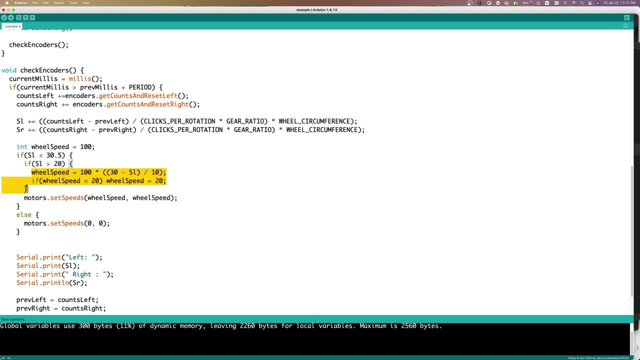 that's going to slow us down right as we approach the end. Now, what's going on here? So I have another if check here where I'm now looking to see. well, we're in our less than 30.5,. 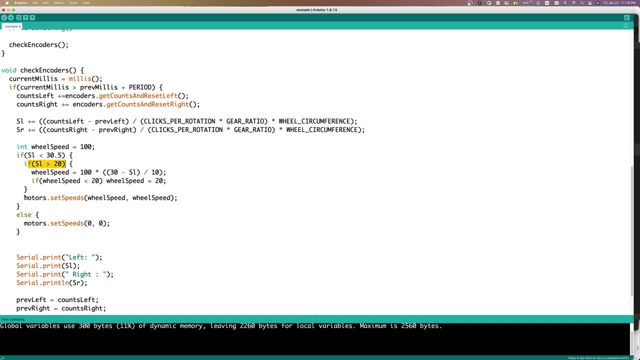 but are we greater than 20?? Because if we're not, then I'm just gonna go ahead like normal and work at my normal working speed. So for the first two thirds of this trip, my robot is gonna continue on its merry way. 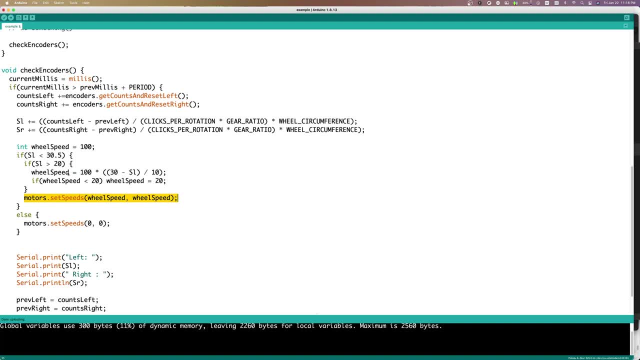 just like it was before, albeit now at half the speed. However, when I'm now within 10 centimeters of my goal, or 10.49 to be exact, I'm going to start reducing my wheel speed. Look at what we have here. 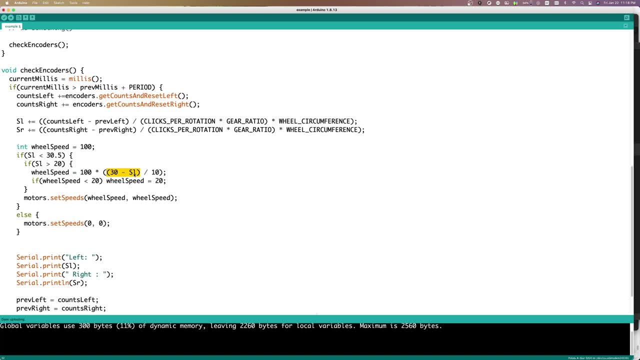 So I'm taking the difference here of the actual encoder value and 30.. So I'm saying: you know what is my actual difference from 30?? If I hit this loop and I was at 21,. let's subtract that from 30. 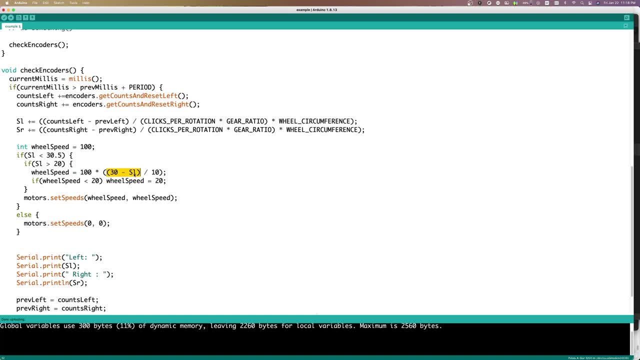 and see that I have nine centimeters left to go. I'm then gonna divide that by 10, so I end up with 0.9, and I'm gonna multiply it by 100 to actually reduce my speed to 90.. So you can see as this goes. 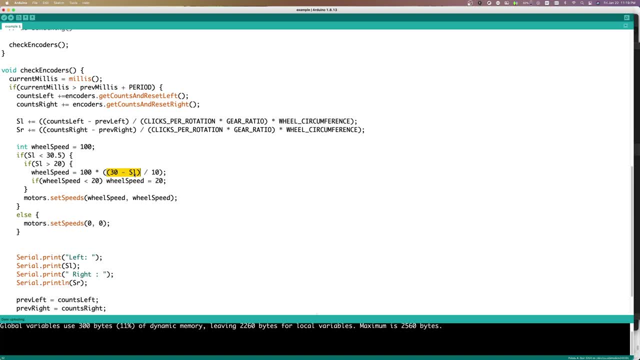 as I'm eight centimeters away, I'm actually reducing my speed to 90.. So, 80 centimeters away, my wheel speed should be 80,, 70,, et cetera. right, This is going to keep going on. 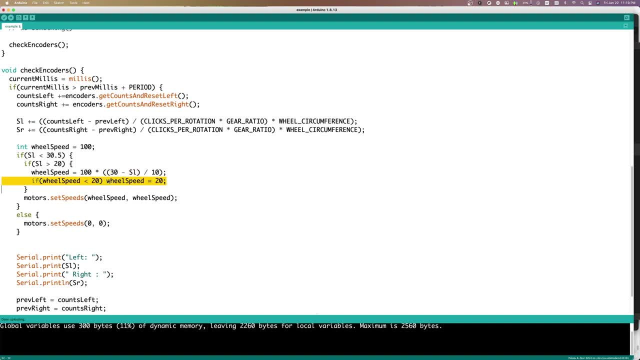 This next line now is to deal with the fact that my robot needs a certain amount of power to keep its wheels turning. If I go all the way to zero, it is actually likely that my robot might fall short of its goal because it doesn't have enough torque to keep itself moving. 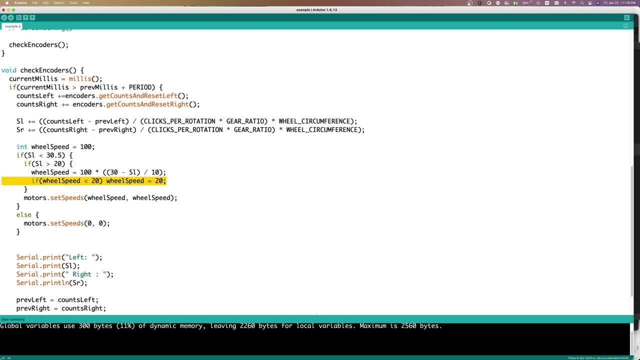 So to try to prevent that, I'm going to reduce my wheel speed. I'm going to reduce my wheel speed to 20, but if it goes below that, if I was, say, only one centimeter away here at 29 centimeters, 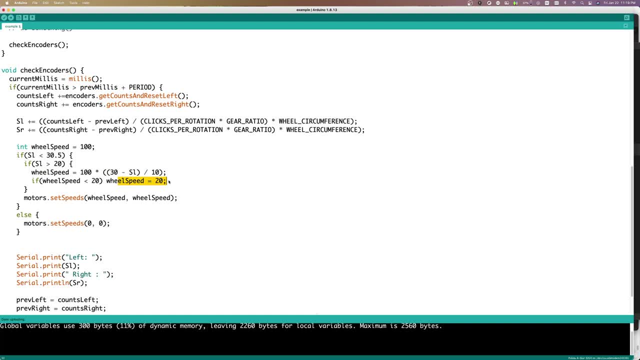 this condition here would automatically keep the wheel speed at 20. It will not go below that. I think this is going to have a good effect, but let's go ahead and see, And I wanna point out that this may require some tuning. 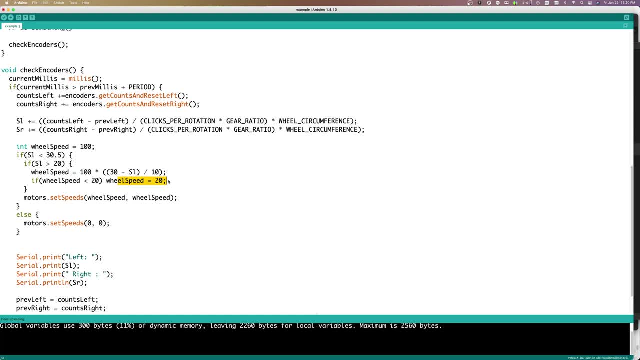 If you have a Turtle Edition or Hyper Edition or any other type, even if your DC motors are different from mine, if your robot weighs more than mine- any factors can change this- You might have to insert your own values. These numbers might not work precisely for your robot. 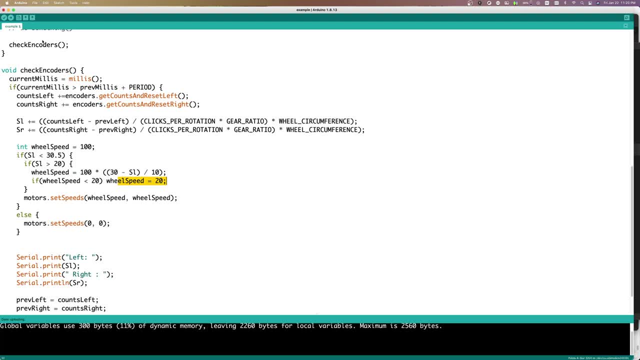 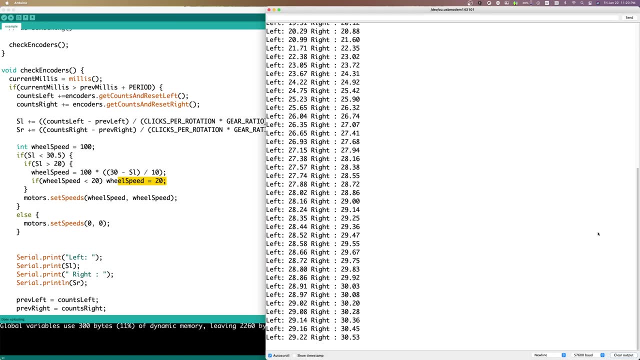 but the idea will All right, let's go ahead and see how this works. Check that we can compile and we can. Let's go ahead and load it up. Look at that pretty close Now. notice the right went a little further than the left. 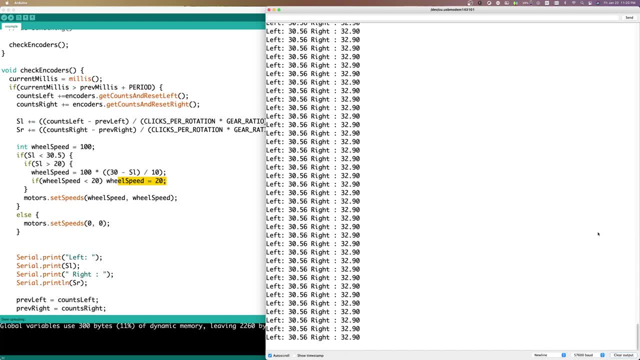 I still have the tether in, since I don't have to reflash. I'm actually going to remove the USB cable and see if that happens again now without it. So I'm resetting it now. Obviously, the serial monitor won't show the difference. 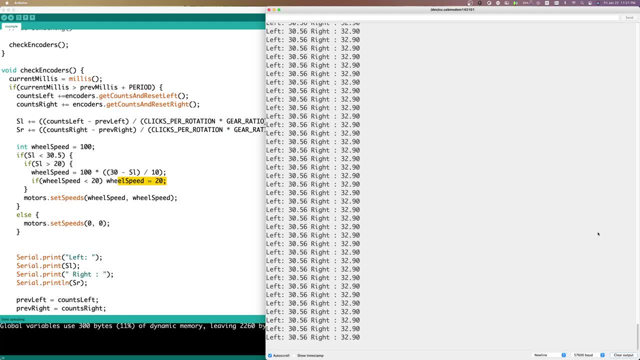 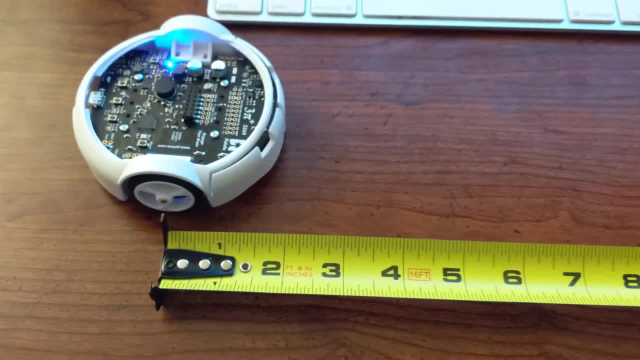 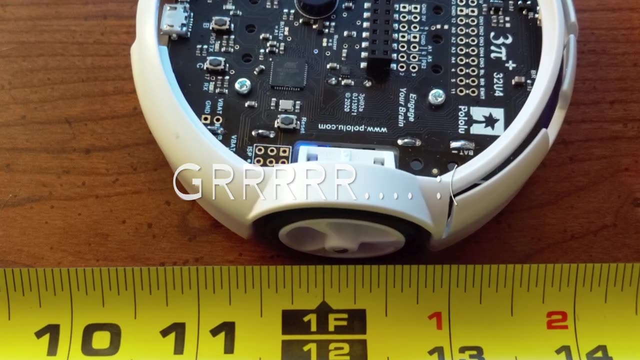 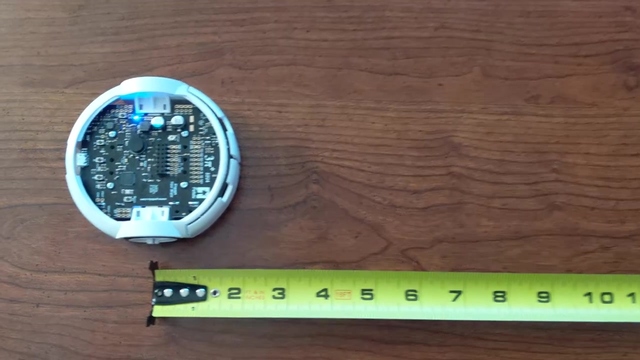 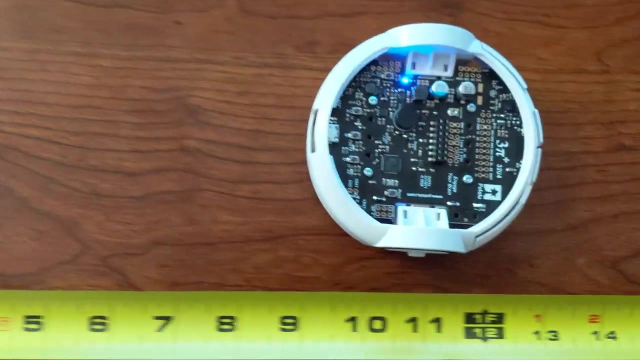 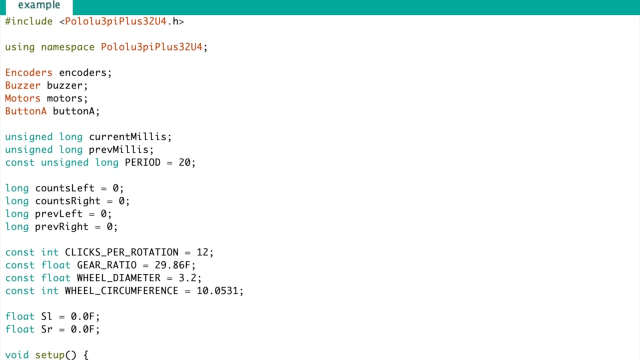 and that looks pretty clean. Let's go ahead and put this next to the measuring tape and see how we do. Congratulations on completing the very first lab in the series. I would like you to think now about how you can take what we've learned here now. 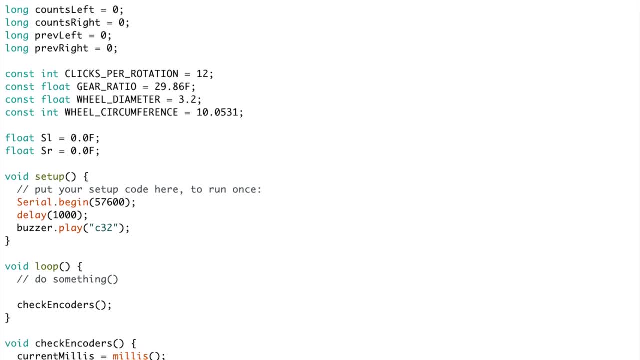 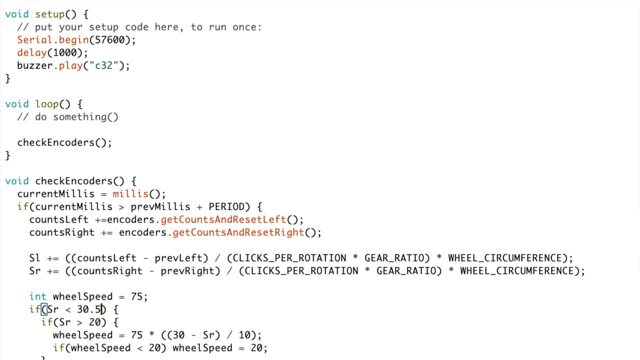 and apply it more broadly. What if your robot wanted to travel faster than 75 out of 400?? What if it was traveling any distance going to a goal where you didn't actually know exactly how far it was going to be away when the robot started? 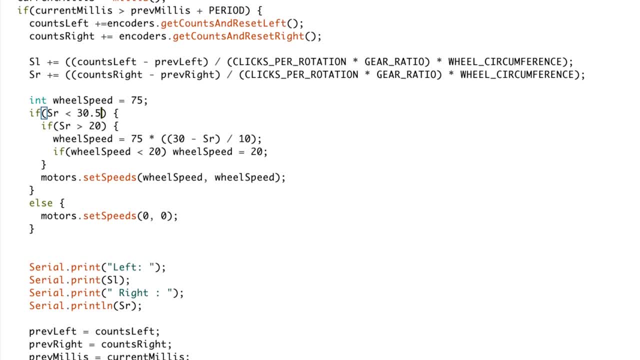 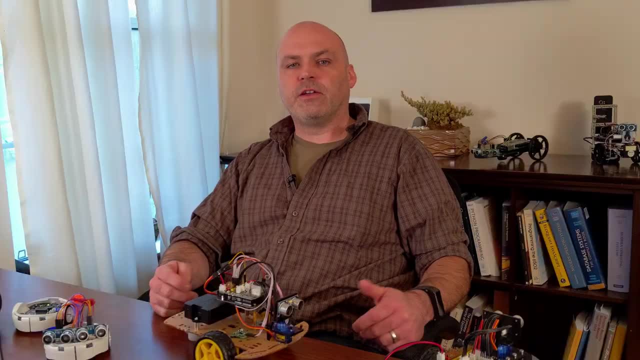 Perhaps you can use it to have your robot navigate a predefined path around your house. Leave me comments. Let me know how you've improved this algorithm, used it and refined it. Thanks for joining me in this very first video in the robotics lab series. 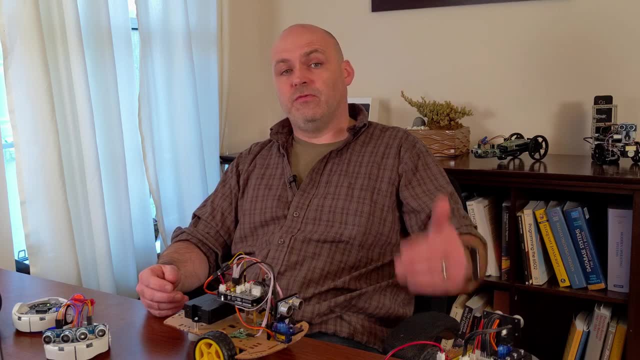 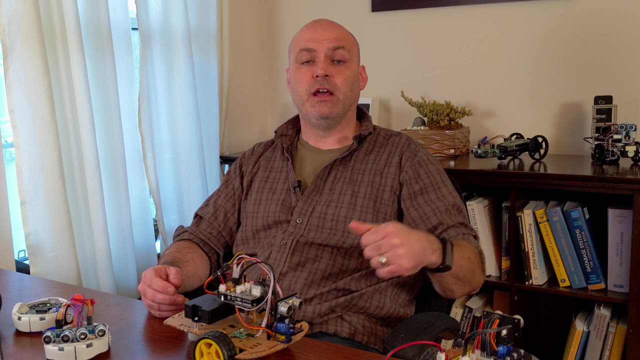 If you like this content, please subscribe. I will be adding new videos to this one. so we're going to be doing PID controller and we're going to be working up to potential fields and path planning. There's going to be a lot more coming. 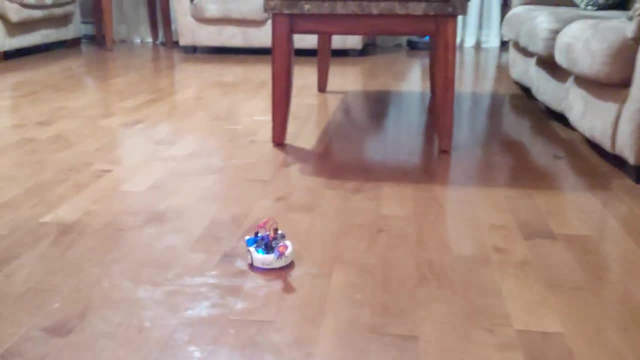 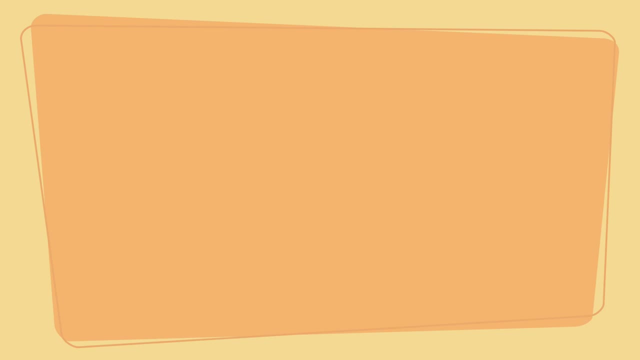 Please do check those out. No robots were harmed in the making of this video. Thanks for watching and I'll see you in the next video. 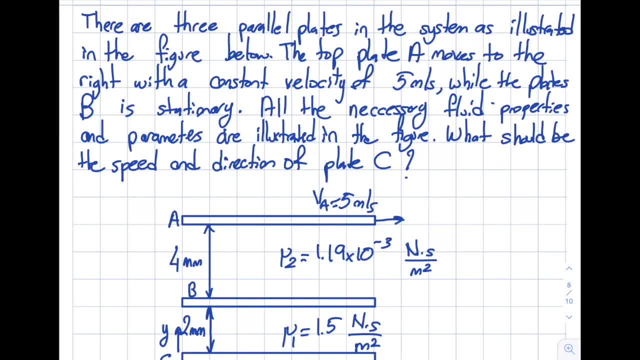 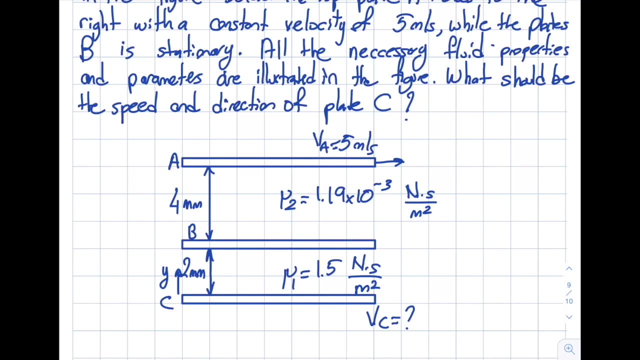 Okay, let's go ahead and solve. whenever we discuss the problem, There are three parallel plates in the system, as illustrated in the figure below. The top plate is moving to the right with a constant velocity of 5 m per second, while the plate B is stationary. All.